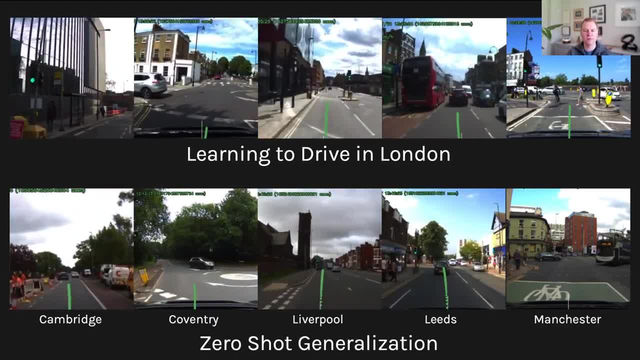 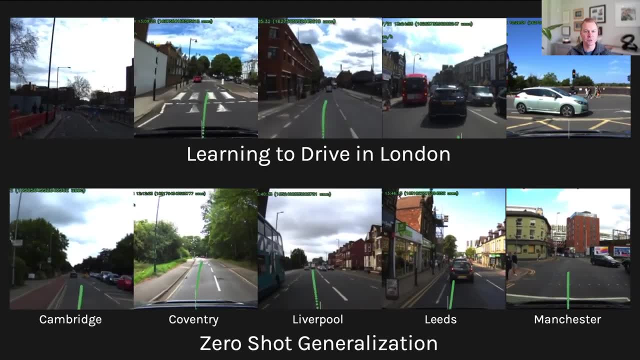 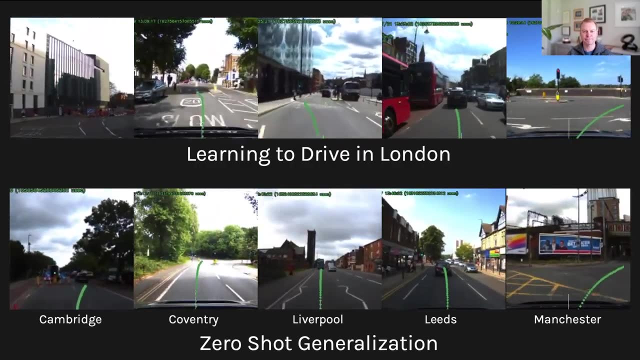 it never had seen these. it didn't have any hd maps of these areas but we were able to take a policy, trained in london of our av 2.0 generalized driving intelligence and applied in cambridge, coventry, liverpool, leeds, manchester. since then we've been working on generalizing. 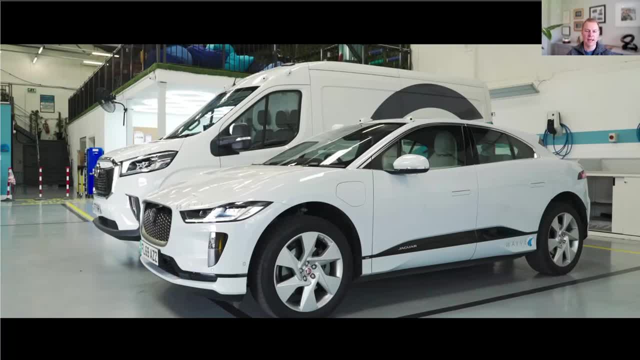 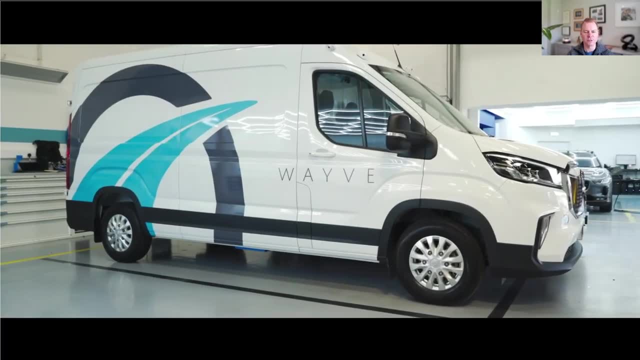 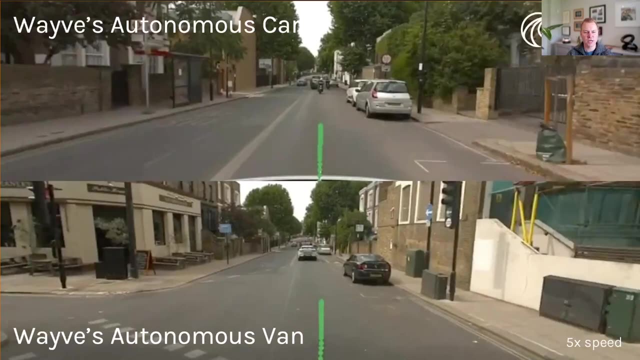 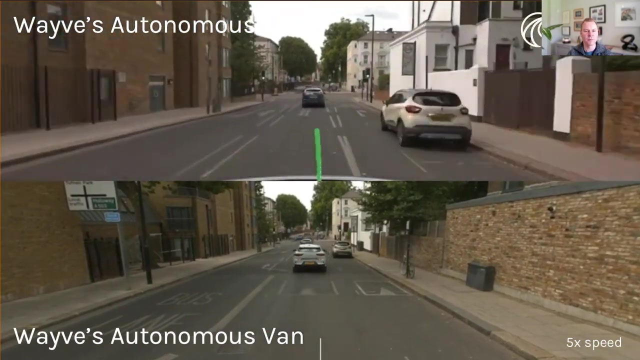 uh, our driving technology across vehicle. and so here is, uh, the, the jaguar ipace that we use and this maxus van that we have built, and again last year we showed that, uh, the same driving intelligence model could generalize across these different uh vehicles. so in this little sped up video you see in the top row, the, uh, the view from our autonomous car. 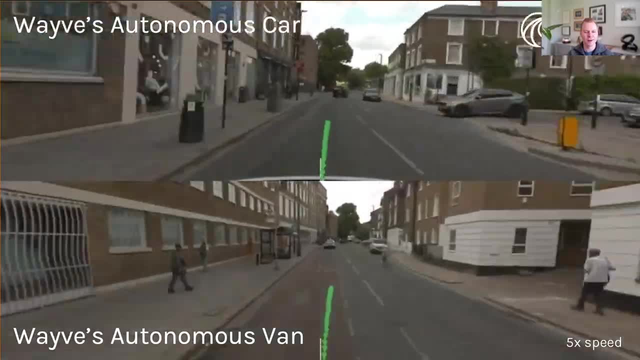 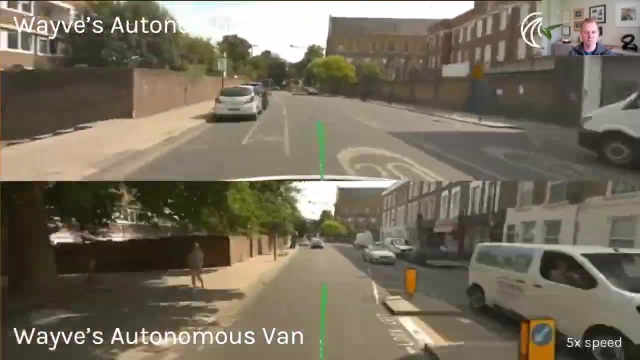 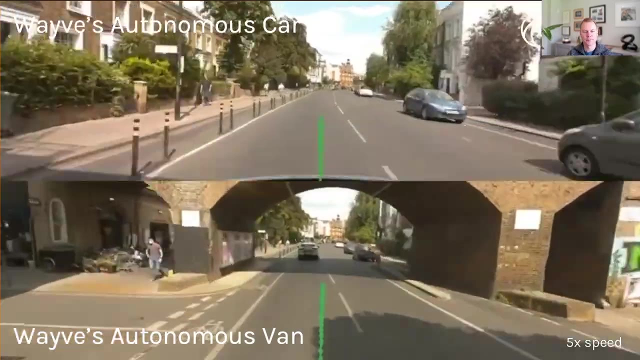 and uh below it. you see the view um from the autonomous van driving using exactly the same uh neural network driving policy, navigating the complex uh streets and intersections of london fully autonomously. we were also very privileged recently to host bill gates, and this is a uh a. 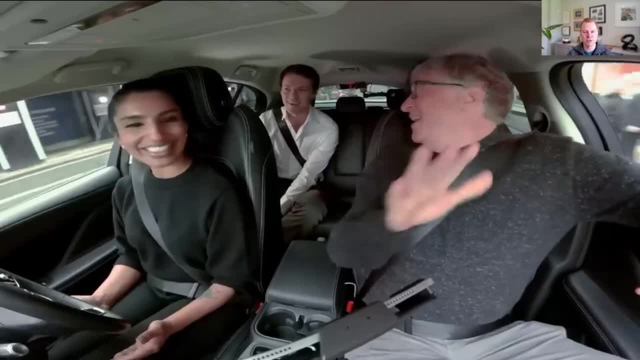 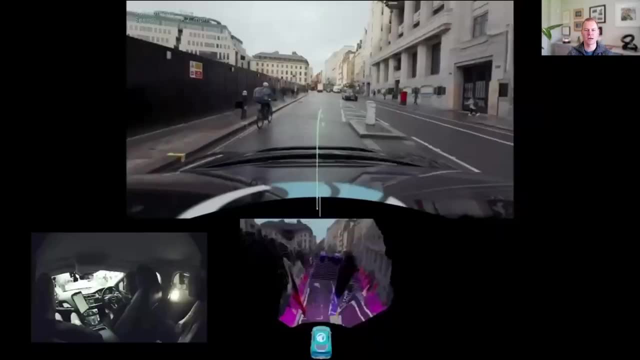 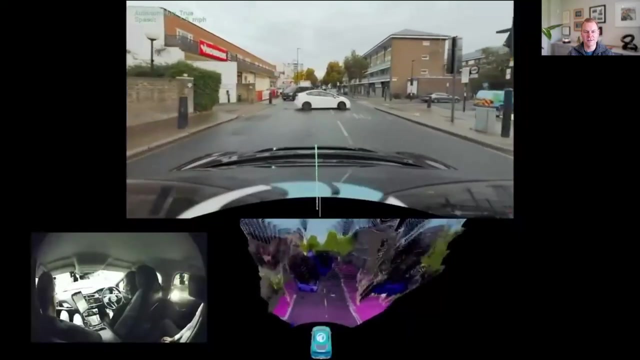 clip from uh the video that uh is out on youtube and you can have a look at in more detail if you'd like. but he had an absolute whale of a time. we demonstrated uh complex driving behavior uh through central london on routes we'd never driven before and uh the seeing you know pretty. 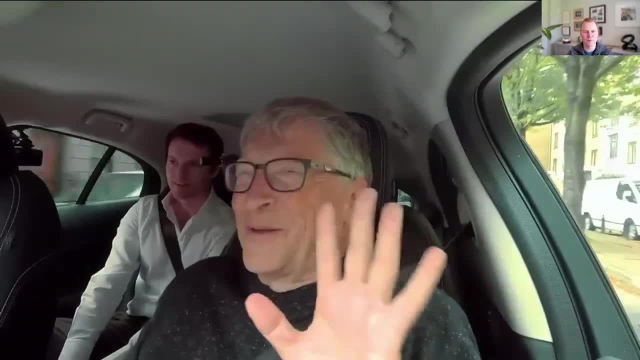 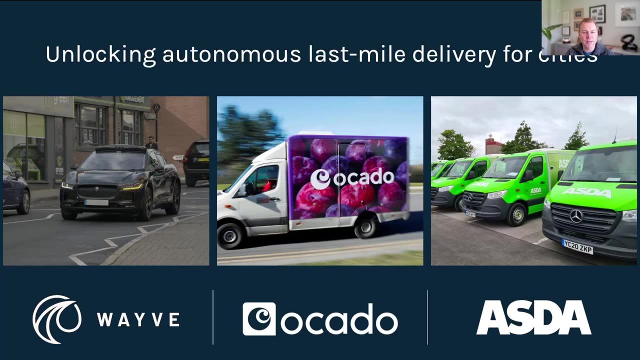 intense and complex uh scenarios such as what we just witnessed there, and more recently, we've uh been working with our partners ocado and asda and just launched a few weeks ago, an actual autonomous driving delivery of groceries in london with asda, and one of the unique things about that is it's 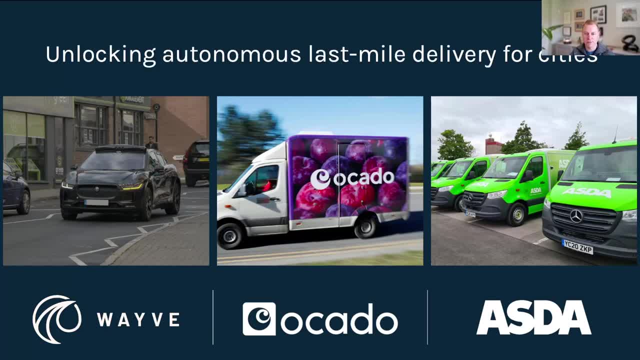 a very large set of postcodes in the uk, so unconstrained. odd, we do still have a safety driver in the vehicle for now, but it's very, very exciting to see this technology be able to scale in a way that supports asda's business without them needing to completely change how they operate. 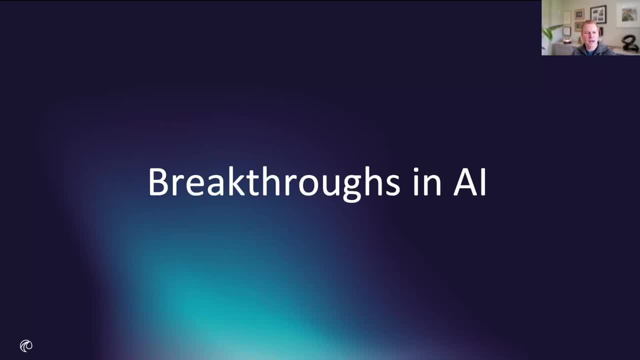 i want to spend a few minutes thinking about, uh, stepping back for a moment and thinking about the breakthroughs we've seen in ai over the last few years. it has been really a phenomenal time in ai and very, very exciting, and breakthrough after breakthrough has come, and i want to think about where this is coming from. what's what's been driving? 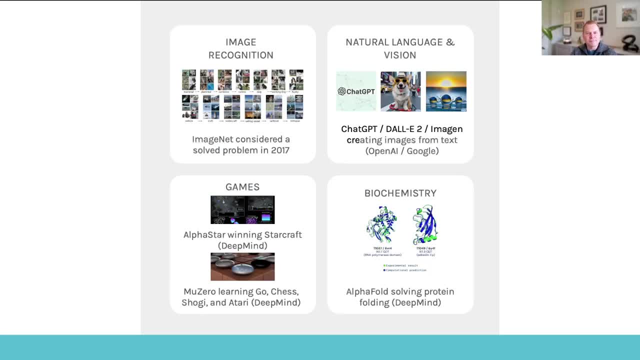 this um, before we do. i mean, you know, you all know these right. uh, the ability now, where imgnect is considered a solved problem, where chat gpt is talked about everywhere by everyone, not just people in ai, where you know big, complex games that were believed to be beyond, uh, computers are. 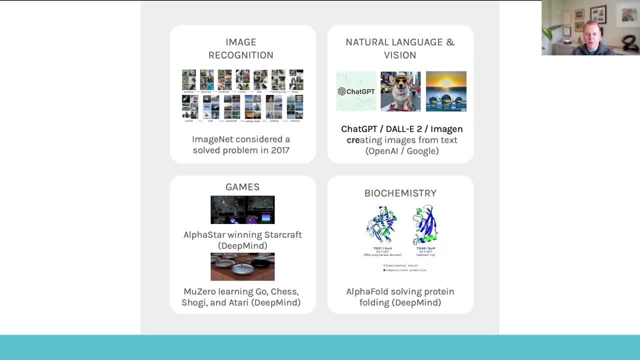 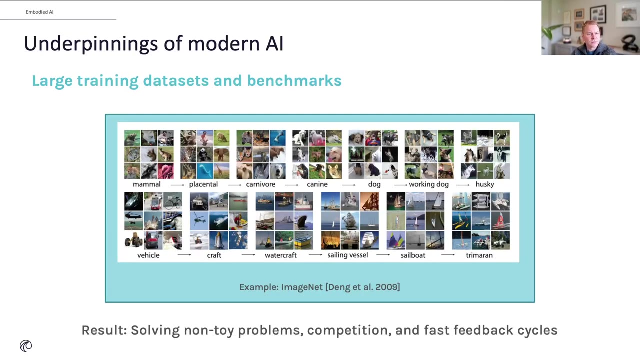 falling game after game, and where we see the the protein folding problem completely solved with a, with things like AlphaFold. It has been an incredibly exciting time. So what's underpinning this? Well, several things. First of all, I think, large training data sets. 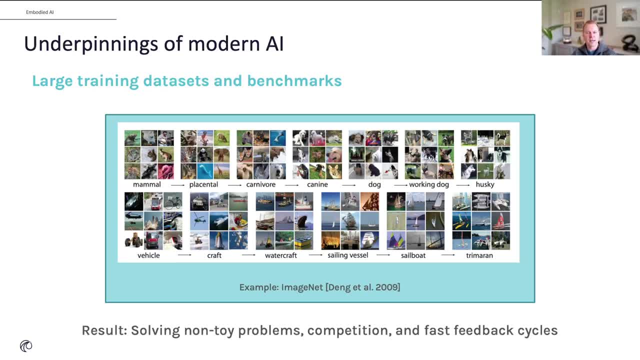 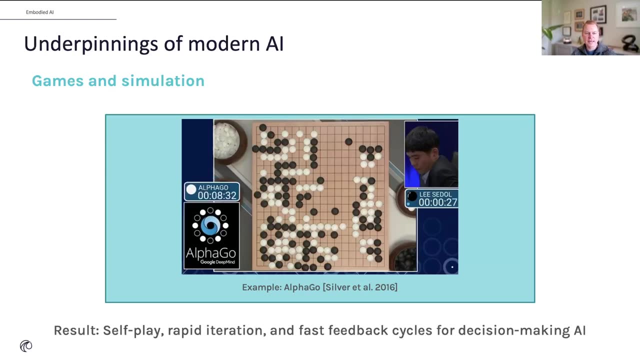 and benchmarks have allowed us to solve non-toy problems. Benchmarks have set up competitions and this has led to a really fast feedback cycle in the community. The use of games and simulation has allowed a lot of reinforcement, learning, self-play- again rapid iteration and fast feedback cycles. 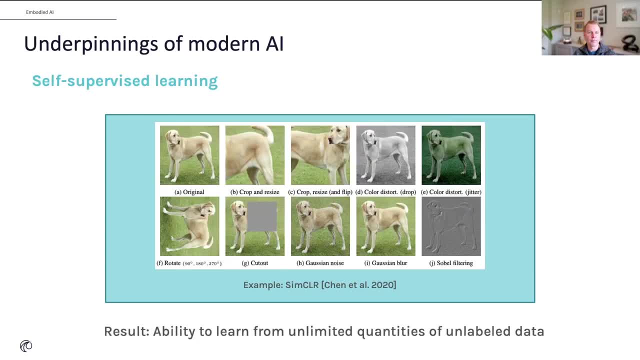 when it comes to decision-making. AI, Self-supervised learning has been a major, major breakthrough of the last few years. that essentially allows us to learn from unlimited quantities of unlabeled data. Previously, you'd have to label this data and that's expensive, slow and constraining. 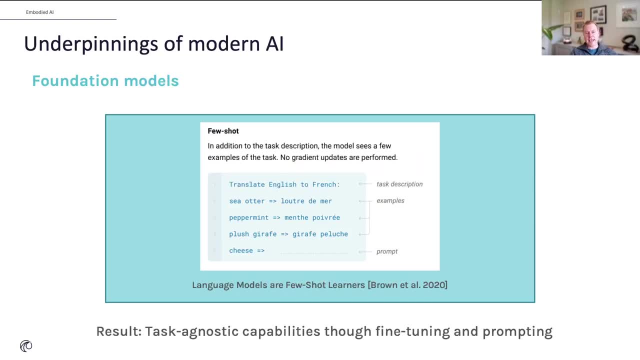 We've seen the emergence of foundation models that take some of those large models that have been trained with unsupervised learning but show that you can use them in task-agnostic ways. You can pre-train a foundation model and then use it, either through fine-tuning or prompting. 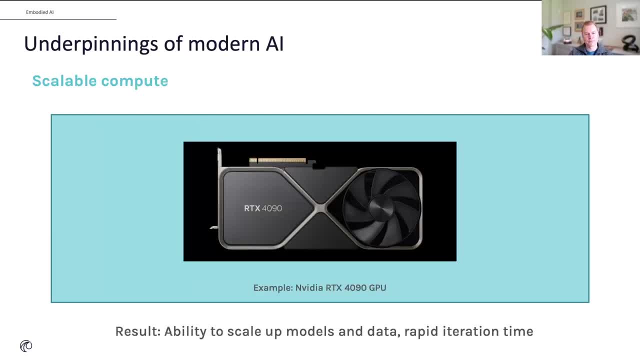 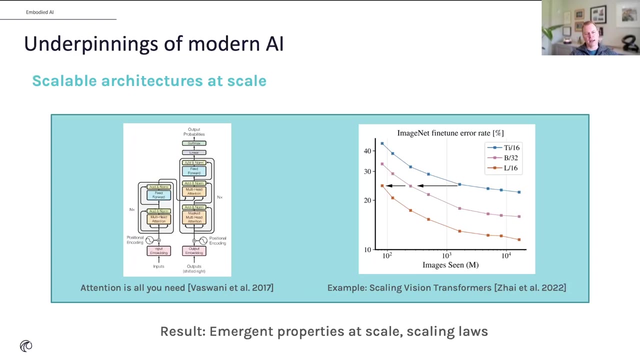 to do a number of different tasks. Of course, all of this has been underpinned by scalable compute that have allowed us to scale up models and data and again iterate fast. But more recently, scalable architectures- transformers, of course, and variants thereof. 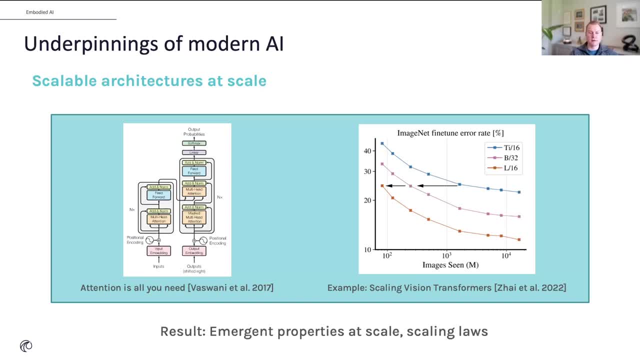 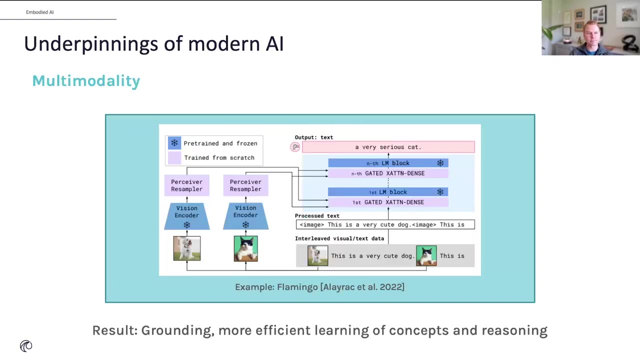 and those architectures being deployed at scale. and then we see things like emergent properties at larger scale and scaling curves, scaling laws that allow us to predict how these models are gonna work as we change scale- Another one that has surprised some people, I think. 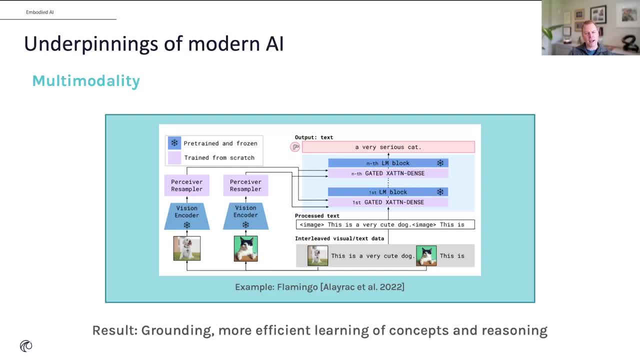 including myself- is multimodality and the rapid use of these general-purpose transformer architectures to be able to bring together different disciplines- NLP, vision, audio, et cetera- and the amazing things that we're starting to see out of that grounding language with images, for example. 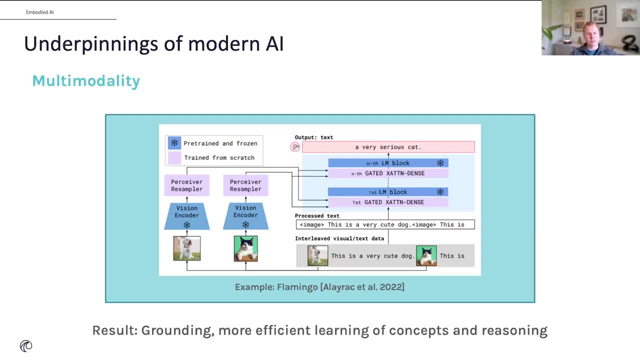 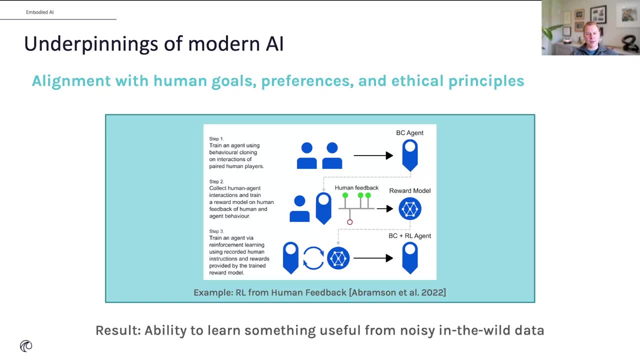 And this also offers really efficient learning of concepts and reasoning. A picture is worth a thousand words, after all, And perhaps the most recent big breakthrough that has really unlocked things like ChatGPT has been the ability to use human feedback to align with human goals and preferences. 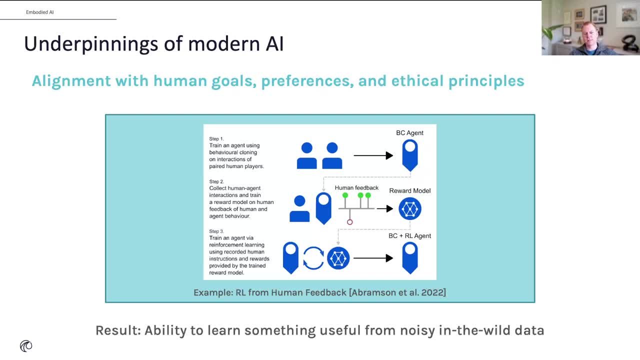 And what this really allows us to do is learn from unlimited noisy corpora of data out in the wild, which on their own are pretty useless, but allow you to learn these concepts and then you can fine-tune those in a way. 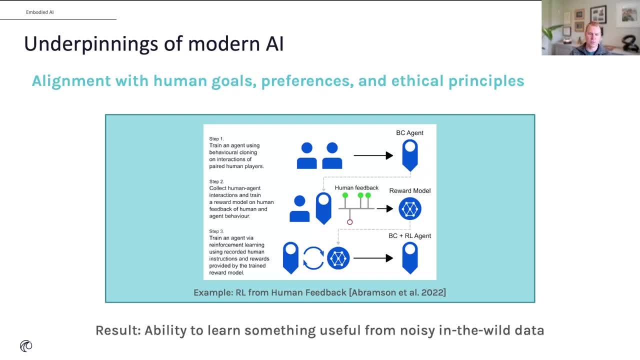 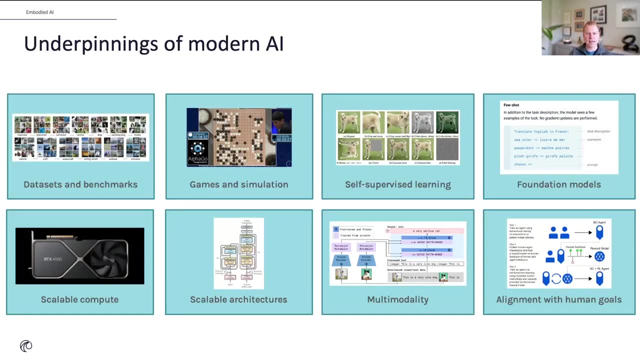 that gives you something actually useful that is acceptable to human use And putting it all together, it looks a bit like this: So it really has been this incredible journey over the last five or 10 years and seems to be accelerating every day. 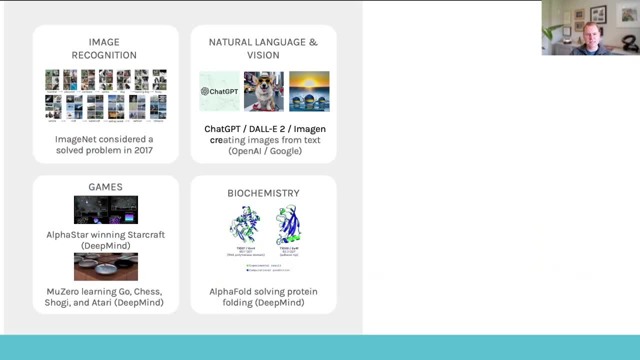 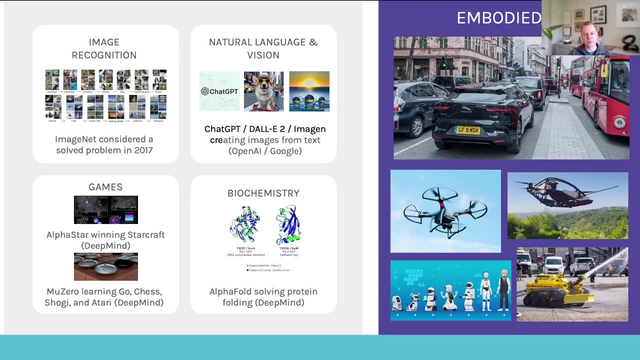 So what's next? I mean, this is what's happened already At Wave. we believe the next major inflection point in AI is going to be embodied intelligence. We are looking at autonomous driving, of course, but there are many, many applications or embodied AI. 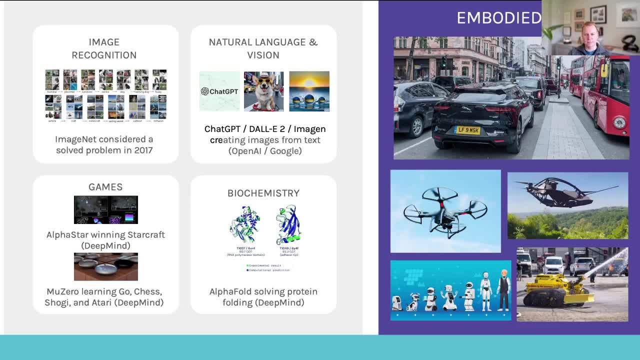 that will require these embodied agents, these robots, quadcopters, et cetera, to have an understanding of how the world works, how it works, to have an understanding of how the world works, how it works, the world works, how things move, how people react to those things, and to be able to deal. 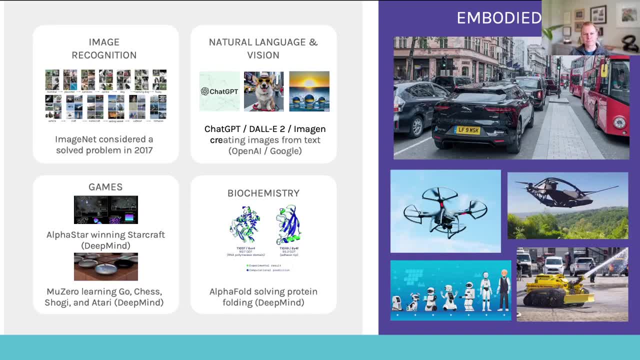 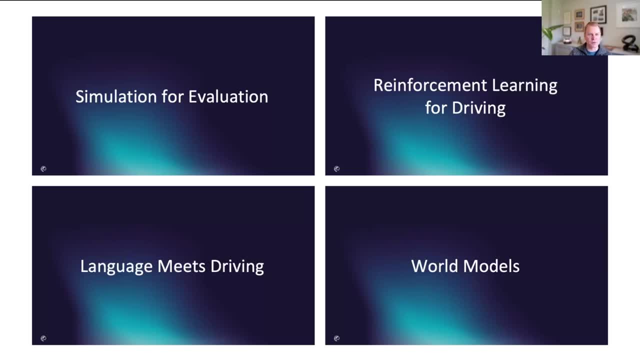 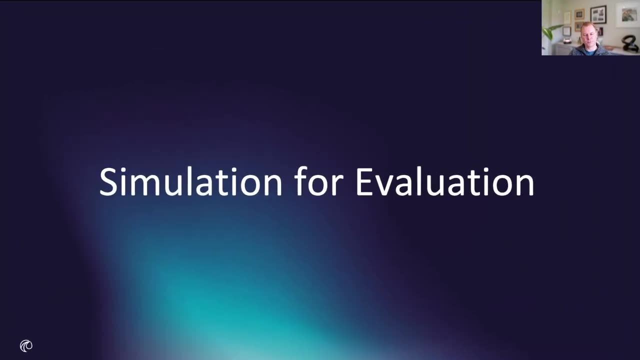 with the open world complexity that's out there. I'm going to talk very briefly about four areas of many others that we're looking at at Wave and some of the exciting work that's going on. So let's start with simulation for evaluation. 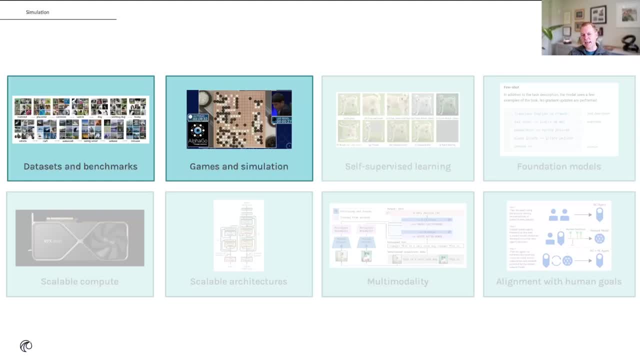 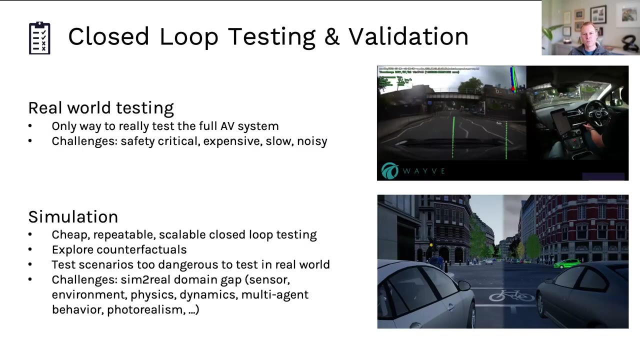 And this really plays on these first two concepts. I talked about the concept of benchmarks that have allowed rapid progress in computer vision and NLP and games and simulation. So when it comes to testing an autonomous vehicle, you can do things like open loop. 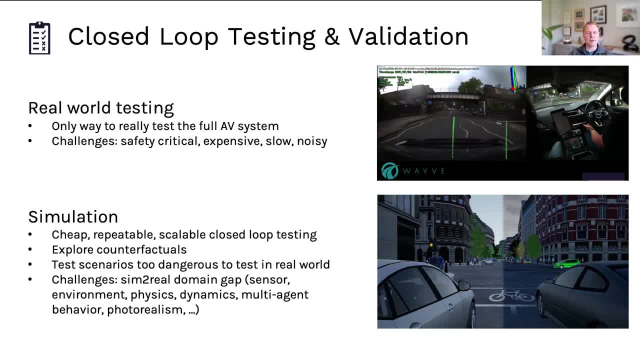 log replay testing, and that does get you somewhere. But really, the thing you really want to know is: how does the system work, And how does the system work And how does the system work In a closed loop? Of course, the ultimate test is real world testing, And that's always going to be. 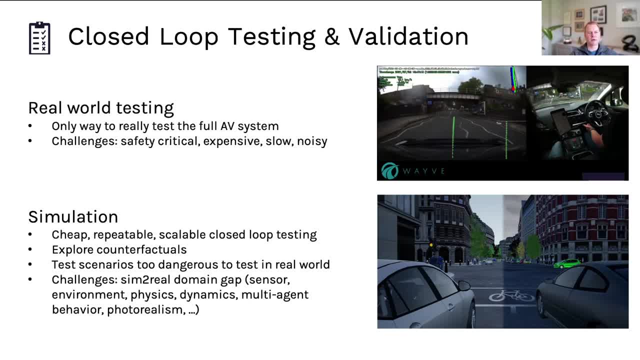 a a an important part of verifying that the whole system works as a whole. But of course this is safety critical. it's expensive, slow and noisy To get the rapid iteration cycle that we've seen in in computer vision, for example. simulation offers a much, much faster test bed to iterate in. 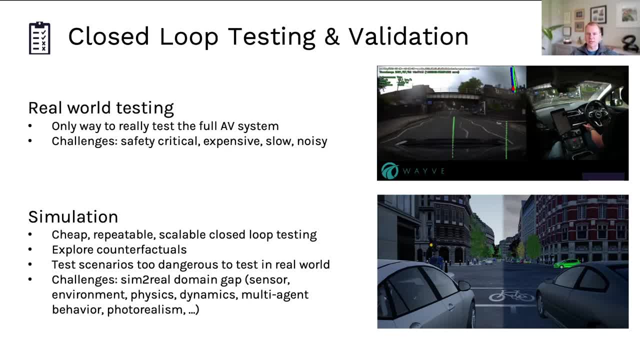 it's cheap. it's repeatable. it's scalable. you can explore counterfactuals. what if something changed in this in the scene? you can test things that are too dangerous to test in the real world. But of course it's got to be realistic enough. you have this domain gap between the simulator. 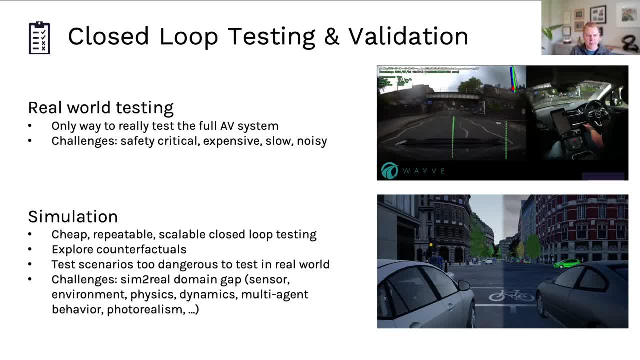 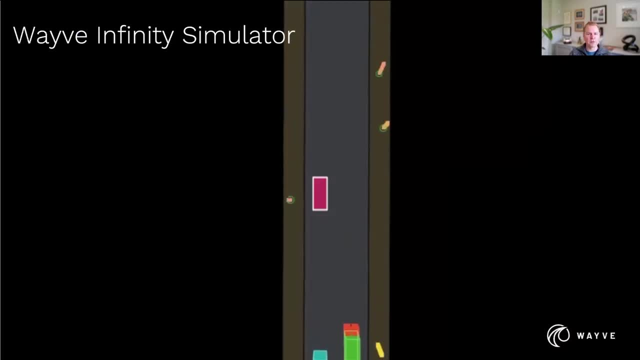 and the real world. And that's not just a visual gap, It's the physics, the dynamics, the multi agent behavior, etc. So it's a it's a challenging problem to get all of that right And that's why we've been working on this wave infinity simulator for the last few years. 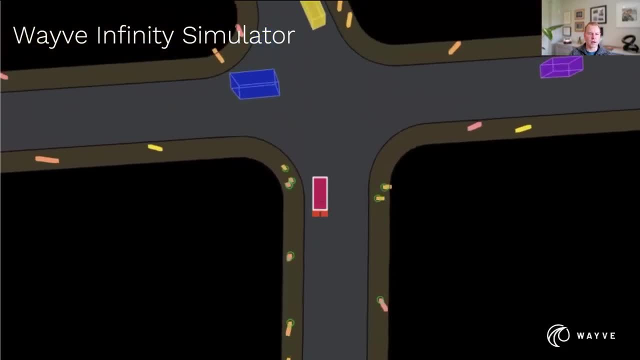 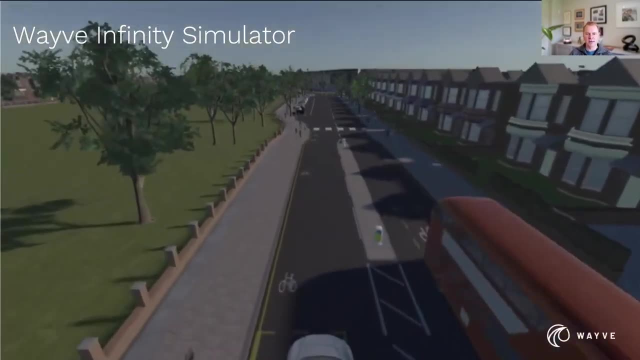 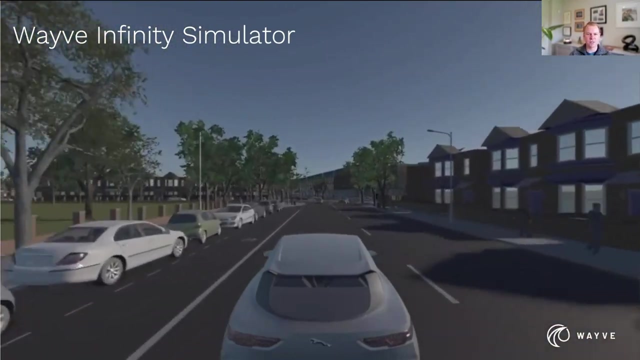 Wave has recognized this and been working on our wave infinity simulator for the last few years, And here's a quick overview. At its heart, it's a fully controllable procedural generation of worlds simulator that connects bird's eye view to full 3d worlds populates that with diversity of 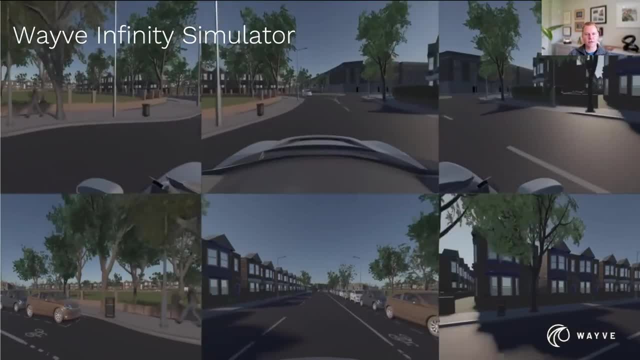 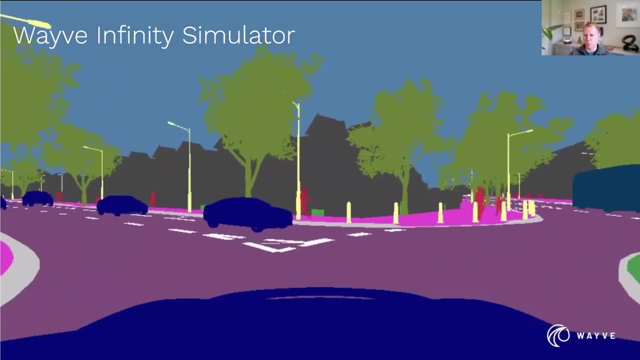 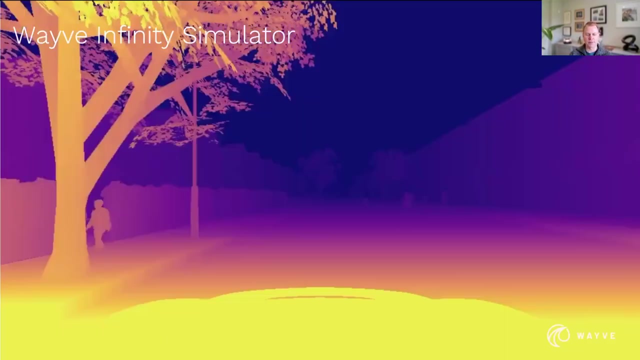 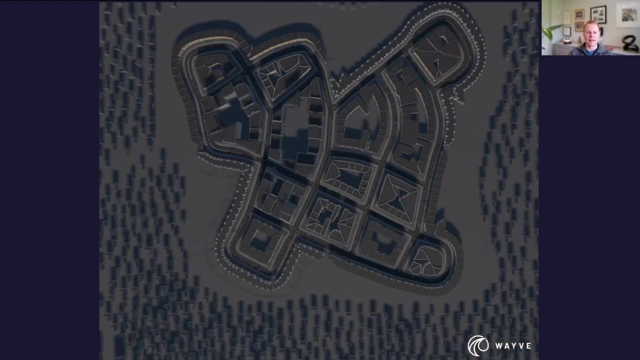 agents targeted at the sort of central London ODD, So we can generate all of the perception inputs that we need from the various cameras And even, if we want to, we can generate these kind of perceptual labels for segmentation or depth, for example. Underpinning this is a generative world creator, And here's a few of the examples. 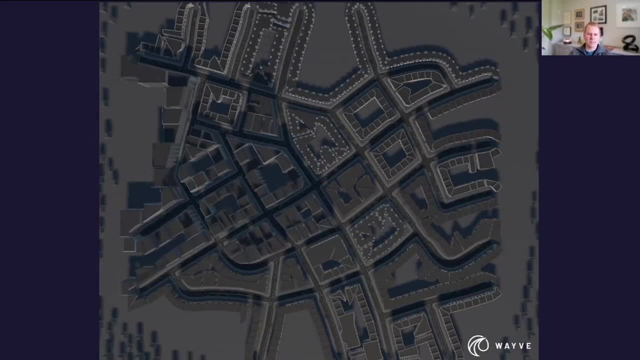 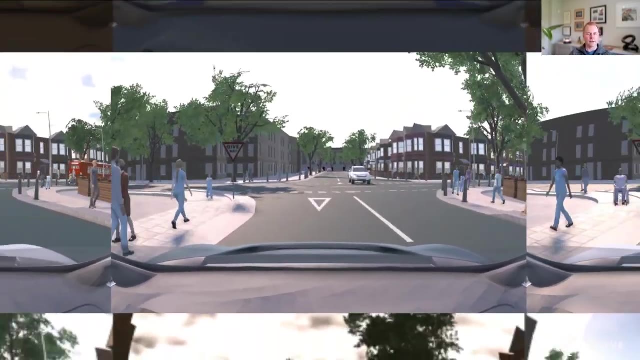 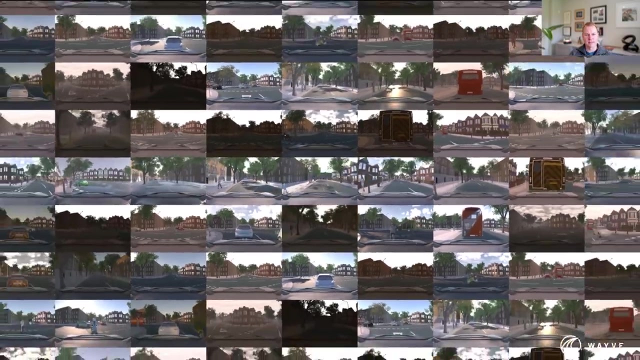 example, worlds that come out of this, And the nice thing about this is we can generate as much data as we want and test as many scenarios as we want, And this allows us to basically be limited by the speed of software in how we test things. Additionally, by having such a wide 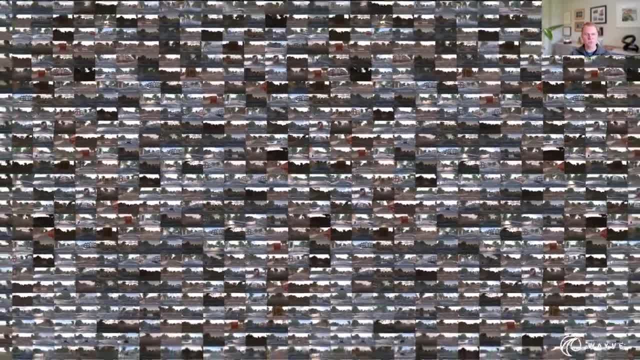 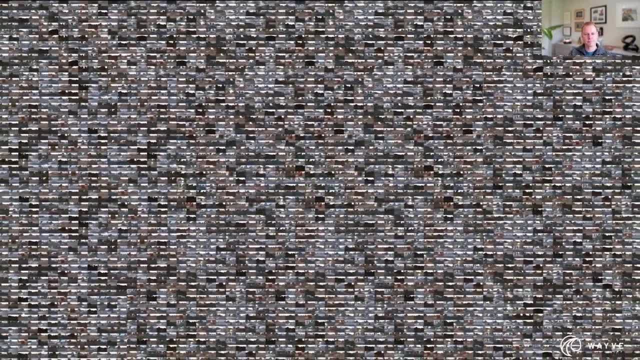 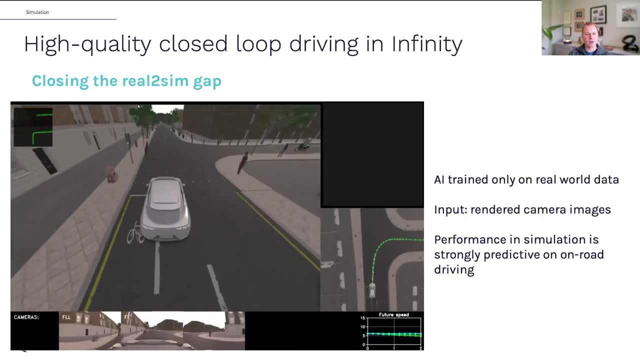 variety of tests, we help. this helps in terms of domain randomization to help reduce that domain gap. Now does it work? Well, here's an example where we have taken one of our driving intelligence models that has been trained only on real world data. 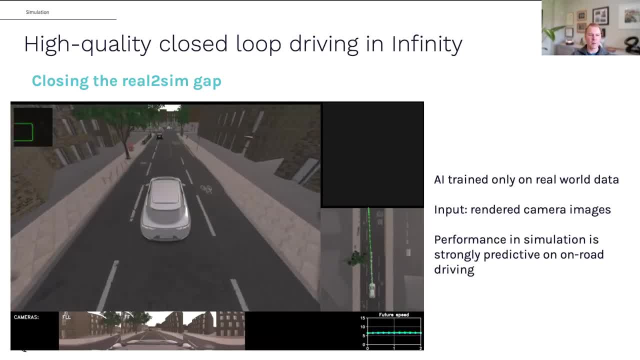 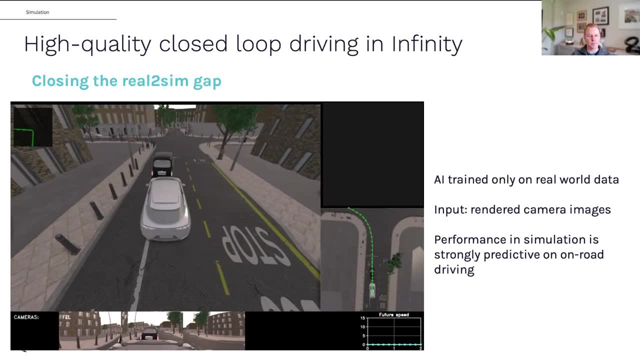 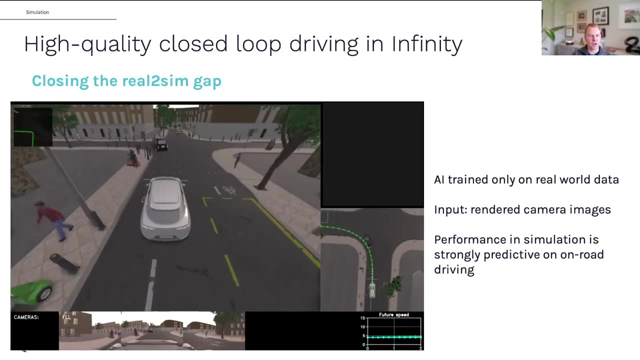 So it has never seen our simulator before. It doesn't know about this. It's experiencing the real to sim gap live, And yet from just the perceptual inputs, the camera inputs that you see on the bottom, it is able to navigate and drive this reasonably complex, busy urban. 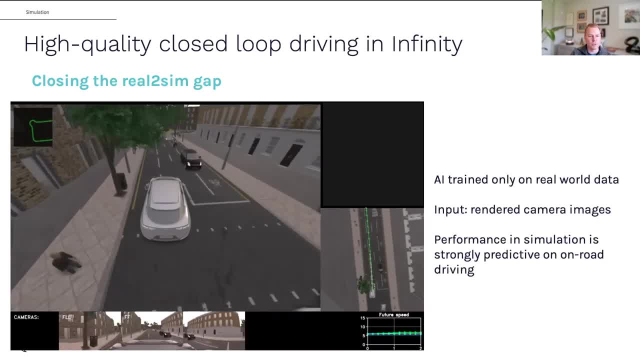 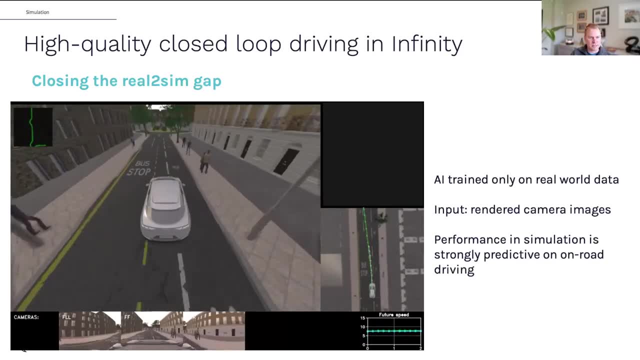 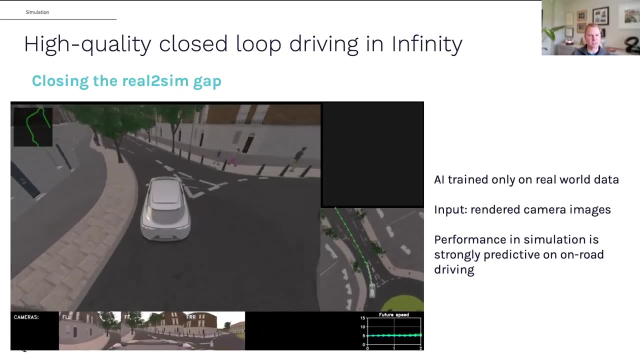 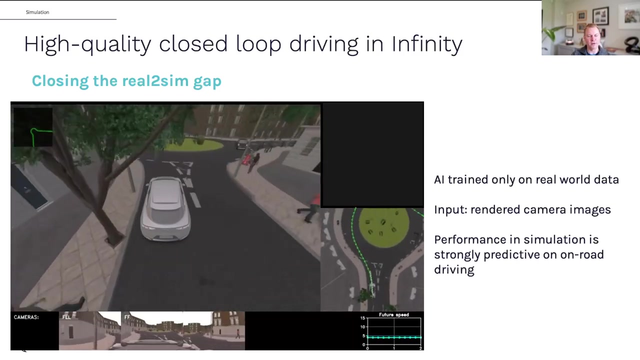 environment And do so for, you know, a significant extended length of time. And what we find by doing this over many such tests, is we get very strongly predictive driving performance in sim that tells us that is a very, very strong indicator of how well this thing would work in the real road. 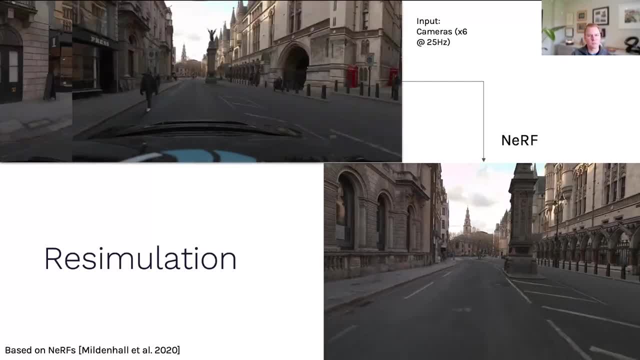 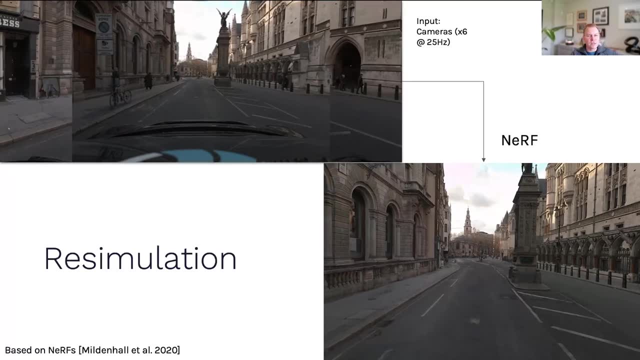 But of course, what I've shown you has does have some clear, very clear visual domain gaps. Another thing we've been exploring is the use of neural radiance fields- nerfs- to re-simulate pockets of the environment. So from a clip, as you see in the 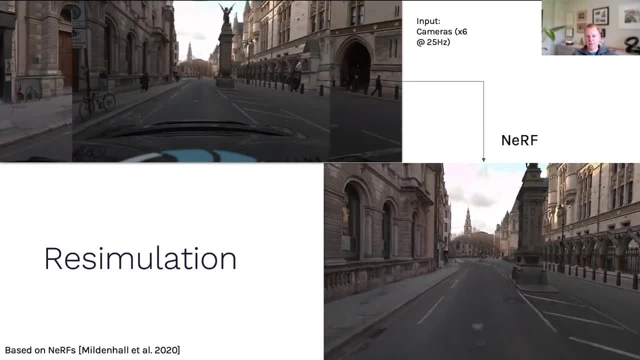 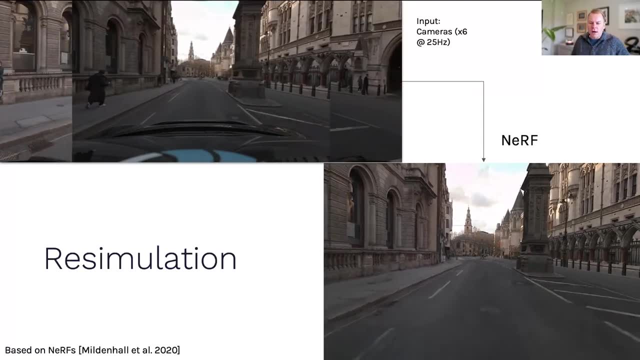 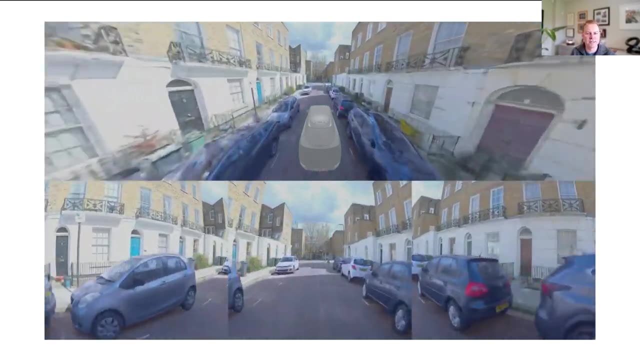 top left of real driving data. we can turn that into the beautiful 3D reconstruction that you see on the bottom right, And from that we can do all sorts of fun stuff. So of course we can replay what the car did. We can do all sorts of fun stuff, So of course we can replay what the car did. 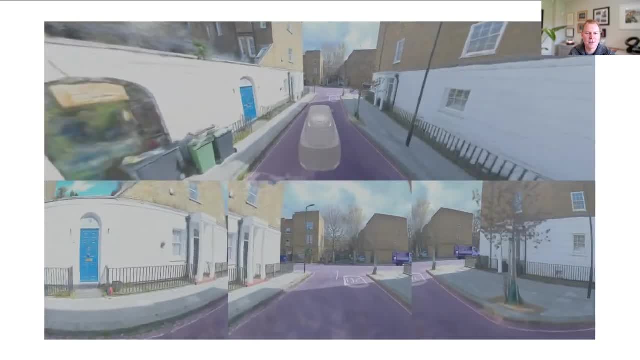 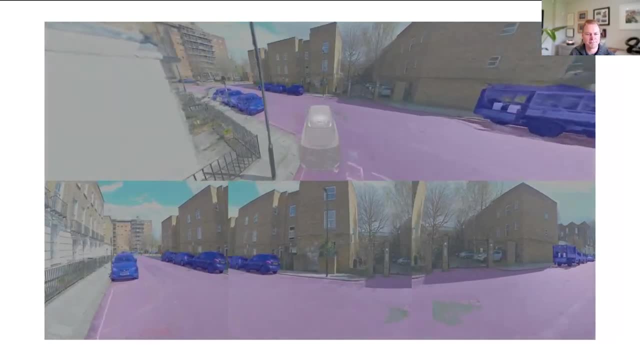 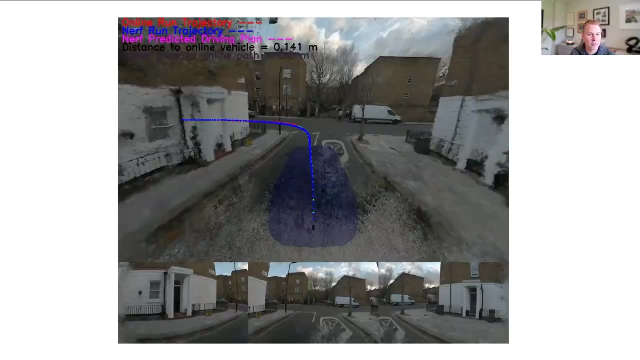 And, furthermore, we can start to use the build of semantic segmentation inside that nerf that allows us to, you know, get this beautiful understanding of what's what. Once we've got that, then we can start to actually replay and again populate this as a simulation. 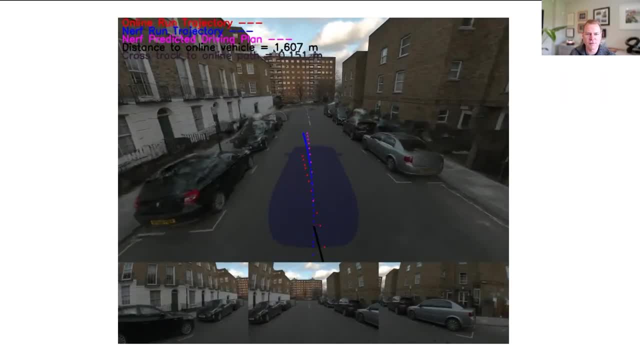 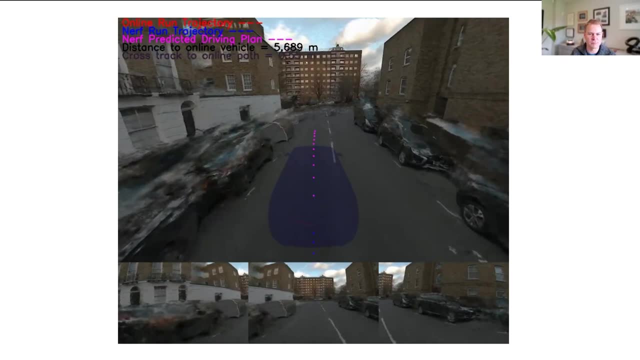 with our real driving models and see how they drive around here, And because we have those semantic segmentations, we can start to apply things in that way. So you know the more you, we can detect things like collisions with the vehicles that are parked here. 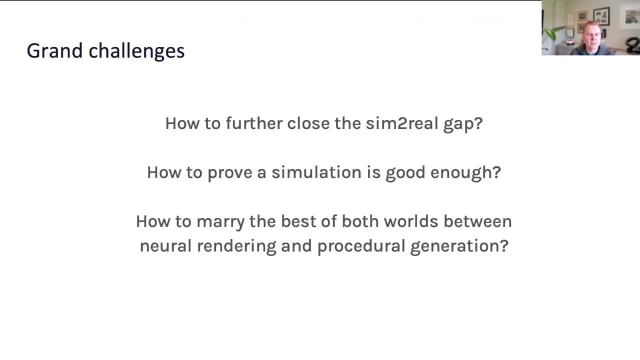 So exciting progress here, but I think there are still, of course, several grand challenges ahead. How do we close that sim-to-real gap, How do we prove that the simulation is good enough, And how can we marry the best of both worlds, between neural rendering and procedural generation? 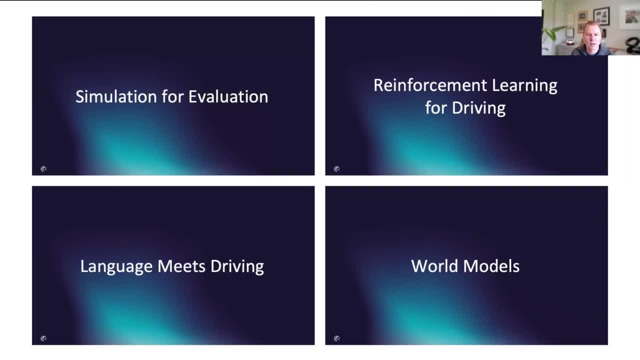 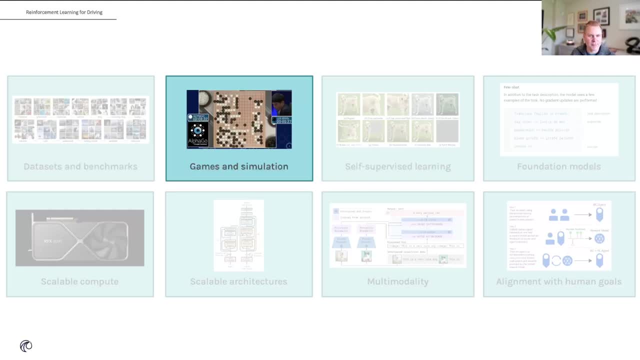 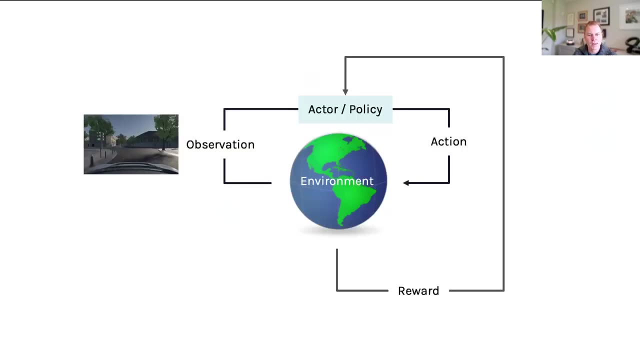 Moving on. I'm going to talk for a few minutes about reinforcement learning for driving, And again back to our menu of AI advances. this is very much aligned with the games and simulation one. Now, I'm sure many of you know reinforcement learning. 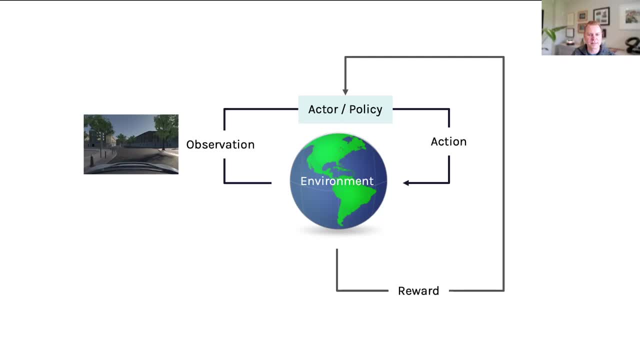 You have an actor or a policy that acts in an environment, it takes actions, it gets observations from that environment and it takes actions from that environment. And it takes actions from that environment And, importantly, it gets a reward signal about you know was that action a good one or a bad one. 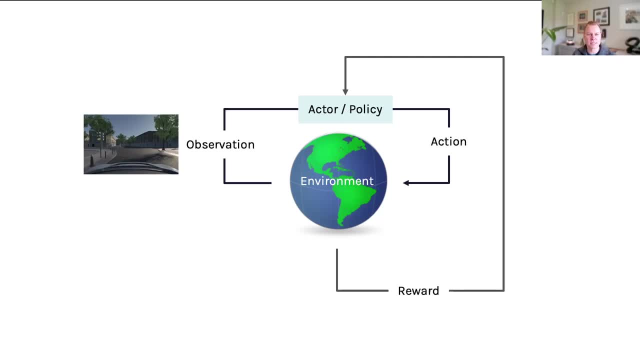 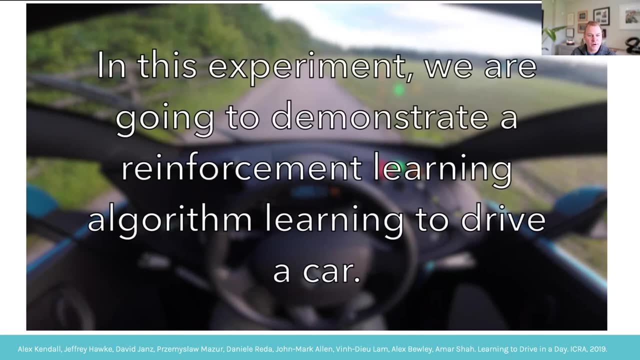 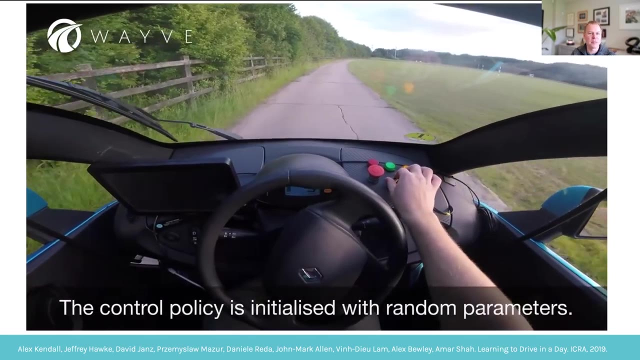 And reinforcement learning is about how do we learn a policy that maximizes our expected rewards over time. Wave actually started very early on exploring reinforcement learning to drive a car And here's a short clip of this where we started on this country road, let the thing explore. 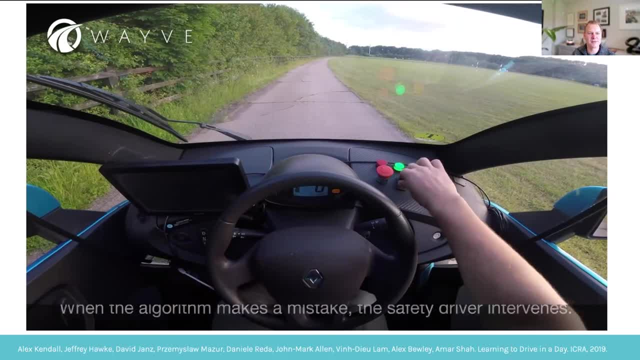 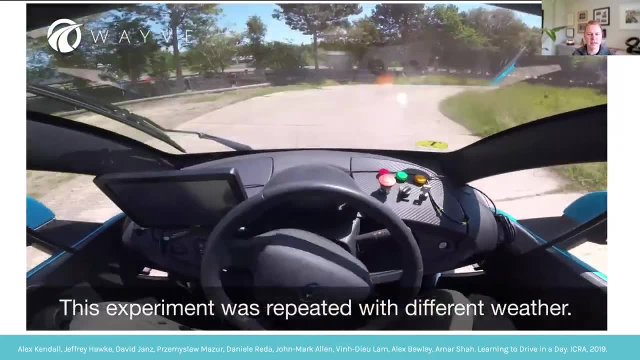 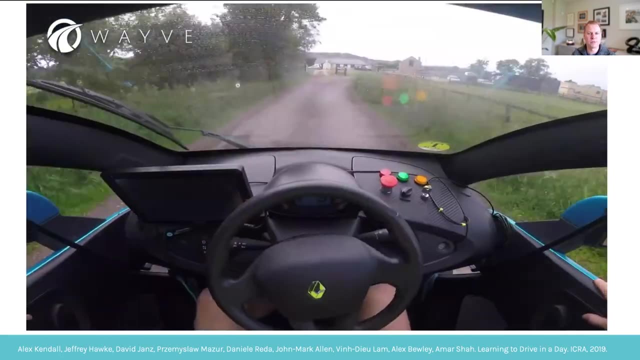 and a human would take over whenever it was about to crash into the wall or run off the road. And if I fast forward the video slightly, you know you get to the end and it's actually able to drive pretty well in a relatively small number of episodes. 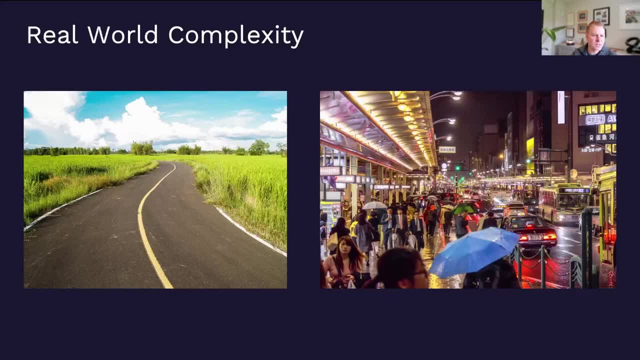 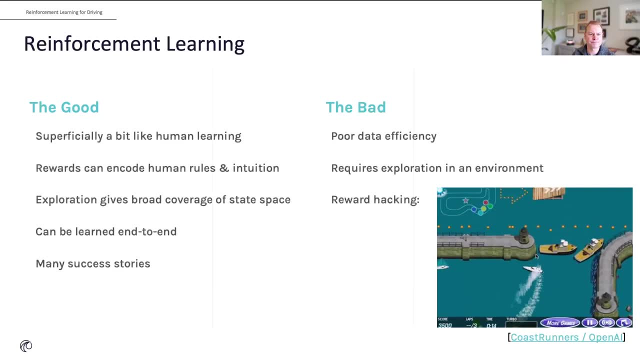 But of course the real world doesn't look like that And what we really care about is being able to act in a busy urban environment. as you see on the right Now, RL has lots of good properties. It's a little bit like human learning, and you can encode human rules, intuition- in the rewards. 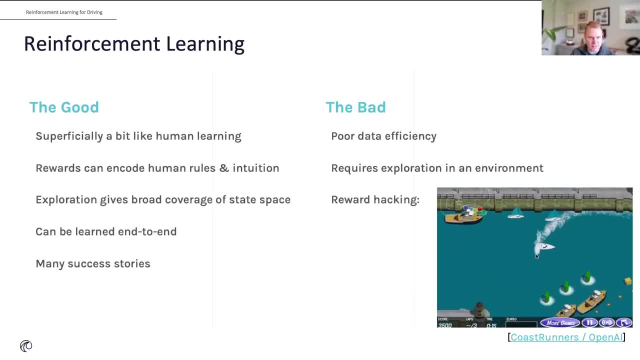 But it is pretty data inefficient and requires exploration in an environment in particular And, of course, in the real world. you cannot allow that kind of exploration that we saw in that early test a moment ago. So how can you get over it? Well, simulation to the rescue. 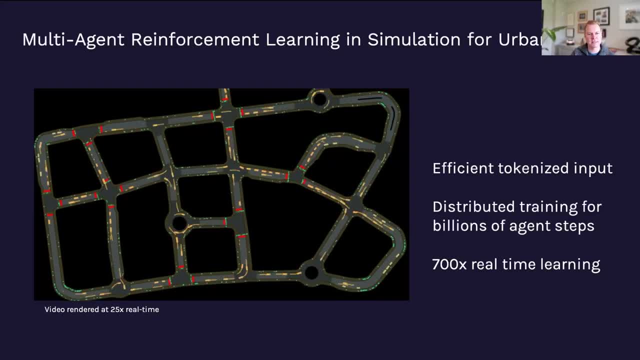 Well, simulation to the rescue. We've been working on multi-agent reinforcement learning in simulation for urban driving for a little while now, building off the Infinity Simulator that I showed you earlier. We're able to learn extremely efficiently about 700 times real time in these dense environments here. 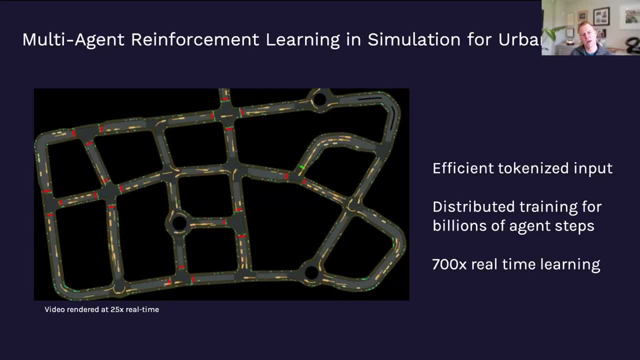 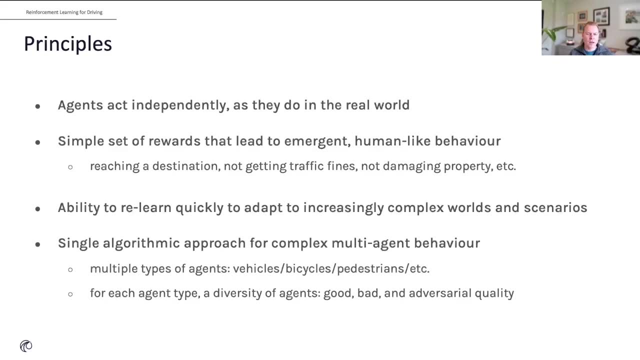 by using a very efficient tokenized input representation and distributed training architecture. As we've gone about this problem, we've had a few principles that we've tried to follow. We want the agents to act independently, as they do in the real world. 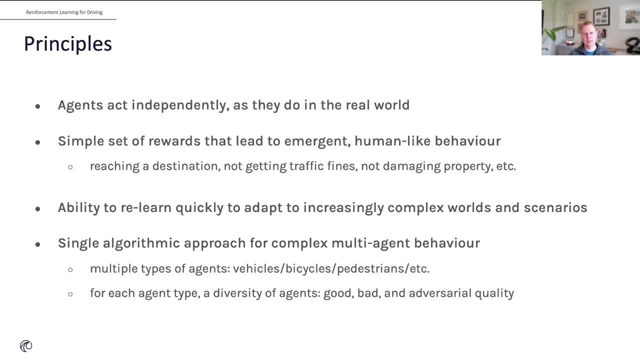 We want to use a simple set of rewards that lead to emergent and human-like behavior. We'll be continuing to evolve the worlds and the complexity of those worlds and the scenarios we want to be able to drive in, And so we need this system to be able to relearn quickly and adapt to those. 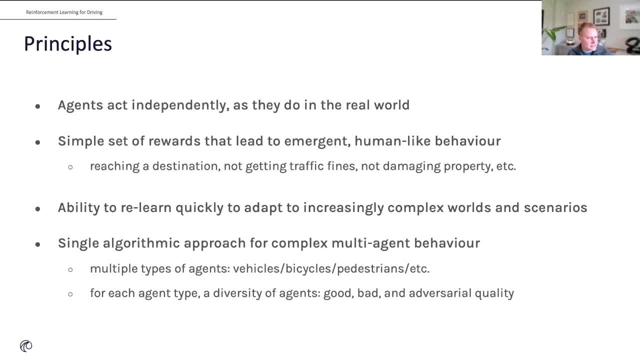 And finally, we want a single system, And so we need this system to be able to relearn quickly and adapt to those. And finally, we want a single algorithmic approach that can result in complex multi-agent behavior, mainly for the ease of development, but because we think it can be done. 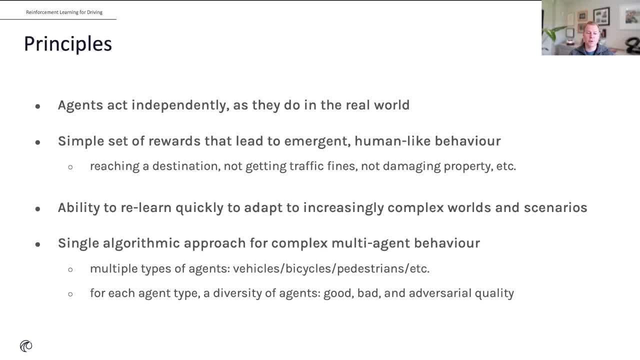 So this includes both multiple different types of agent, but also, for each type of agent, a diversity of agents within that type, both good drivers, bad drivers and potentially adversarial drivers, As I mentioned, one of the keys to the rapid progress of this project. 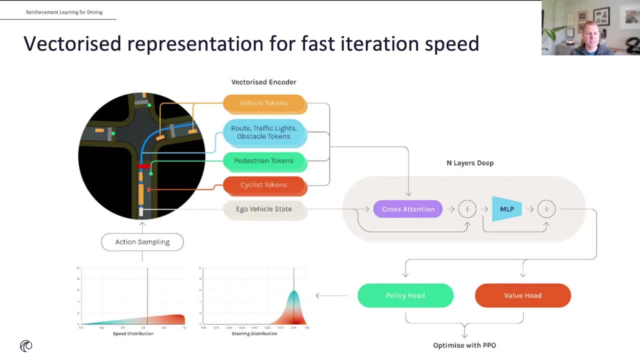 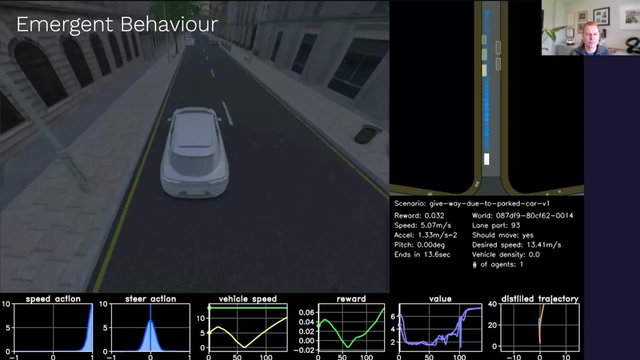 As I mentioned, one of the keys to the rapid progress of this project has been a vectorized representation that basically allows us to learn this thing for billions of episodes in a matter of hours, And that's down to a very, very efficient vectorized representation. 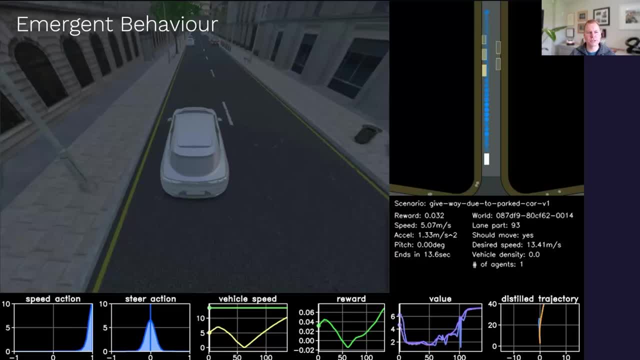 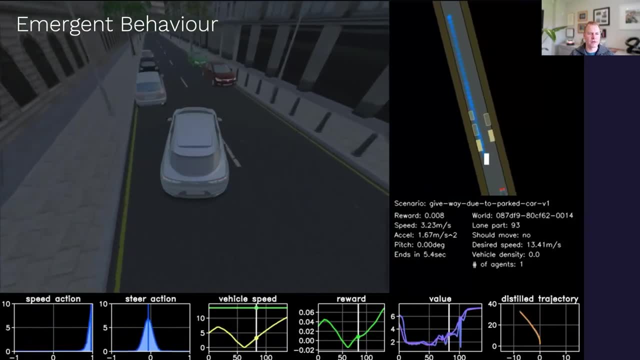 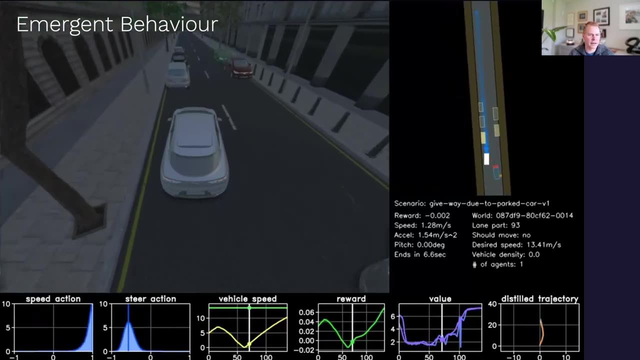 Once you do that, you start to get some really interesting emergent behavior coming out. So here's a video where you'll see the car, the ego vehicle, giving way and waiting for an oncoming vehicle to pass. This is not something we hand-coded. 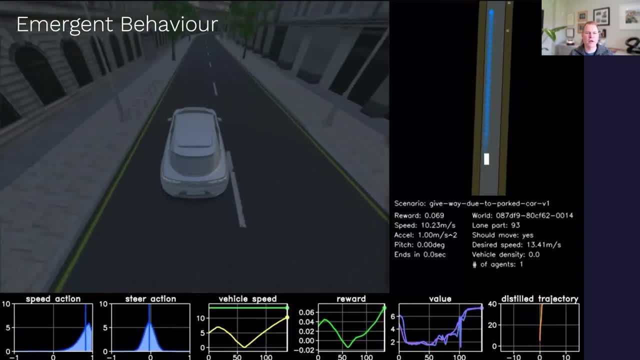 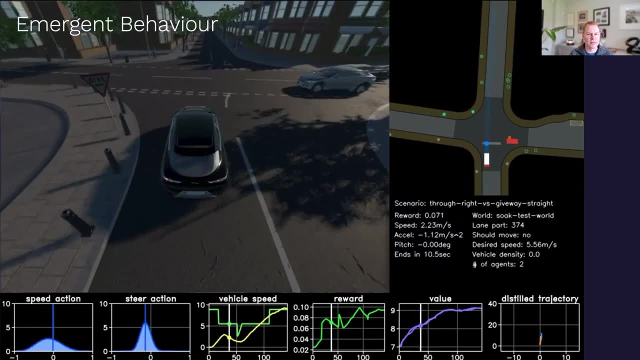 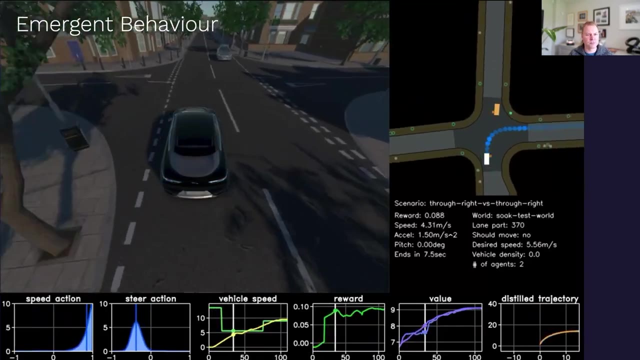 We gave it again: very, very simple rewards of the kind: do not crash into anything and make progress towards your goal. Another interesting example is give-away behavior, And again here's a few different scenarios where the agents have been able to learn. 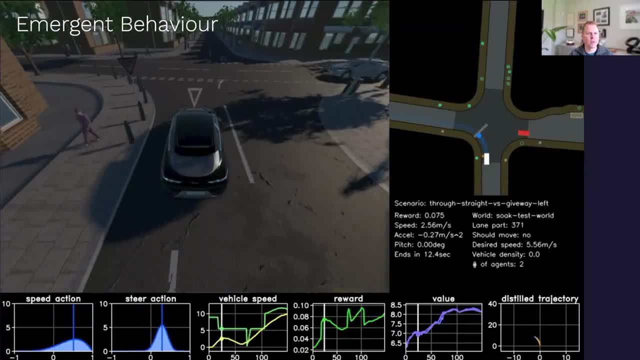 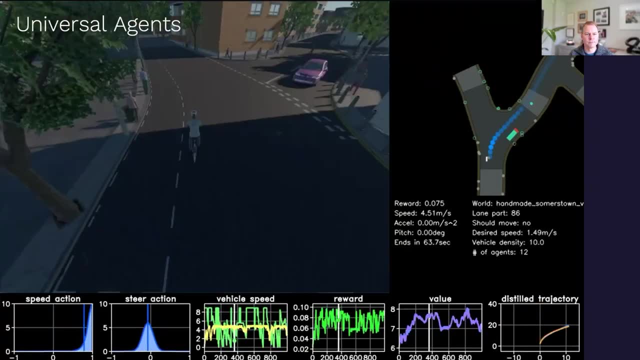 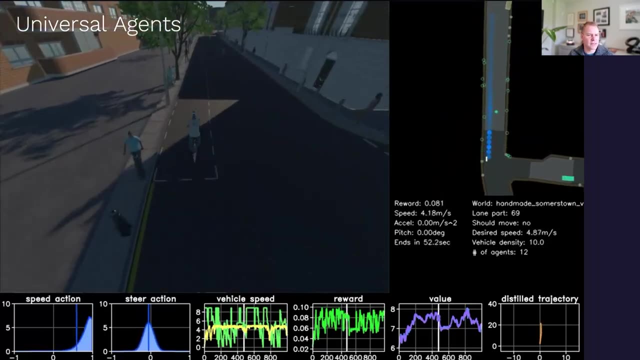 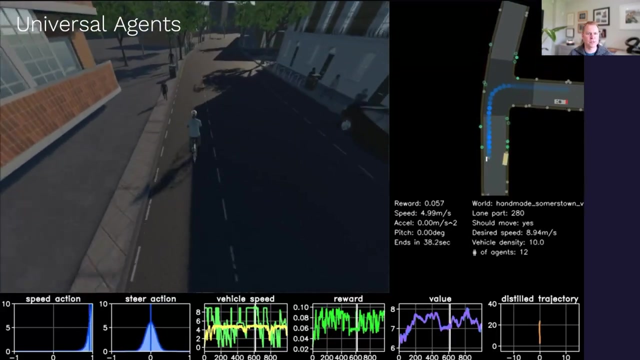 very human-like give-away behavior, again from relatively simple rewards, reward signals. We've also been exploring what we call universal agents, which is basically a single neural network, a single policy that has been trained to be able to act for a diversity of different types of agents. 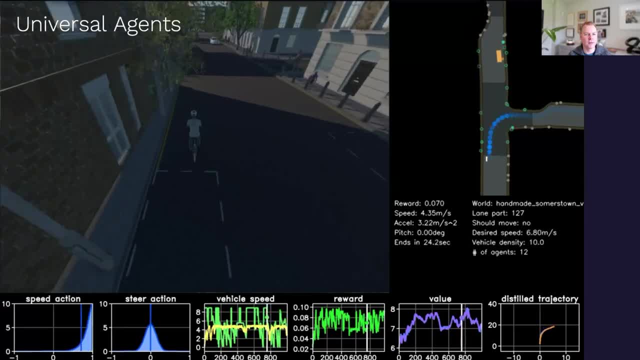 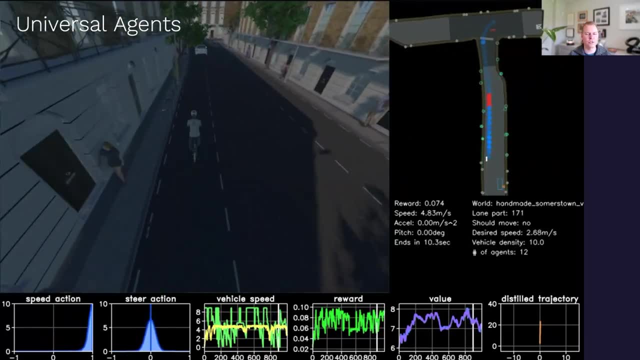 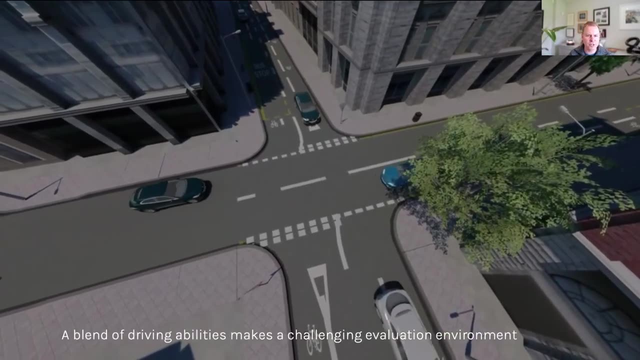 So here, both the ego vehicle and the ego bicycle, rather and the vehicles around here, are being operated by a single driving policy, a single universal agent When it comes to evaluation. one of the interesting use cases of this is actually to populate your world with suboptimal driving. 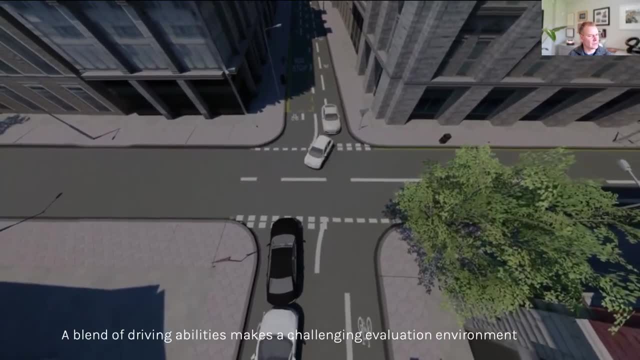 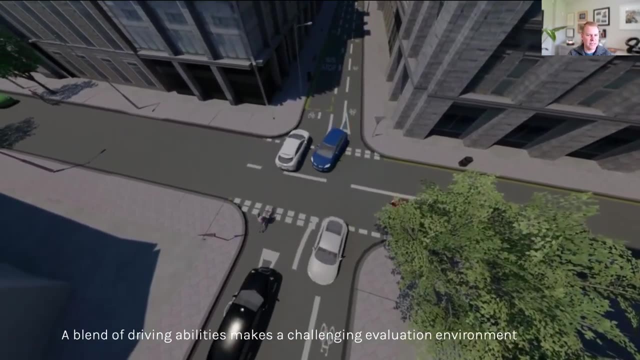 So here's a busy intersection where people are not really following the rules of the road kind of deliberately And you see all sorts of craziness here. Now would you actually see this, this kind of craziness in the world? Well, probably not for the cars. 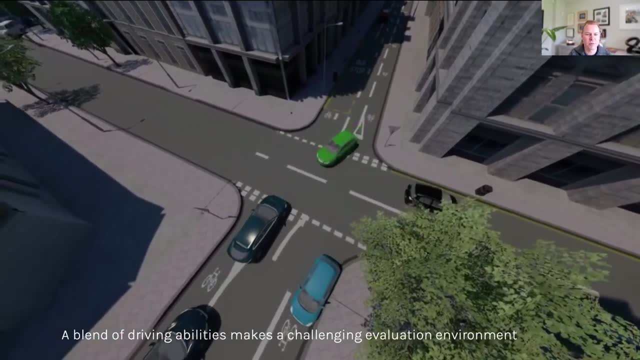 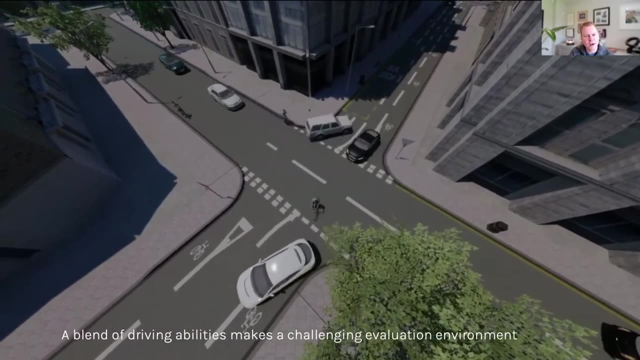 Maybe for the bicycles. That's not that unrealistic for bicycles, at least in Cambridge where I live. But importantly, our driving intelligence needs to be able to cope with those kind of crazy scenarios and be able to manage that, And so it's important that we're able to generate this kind of behavior. 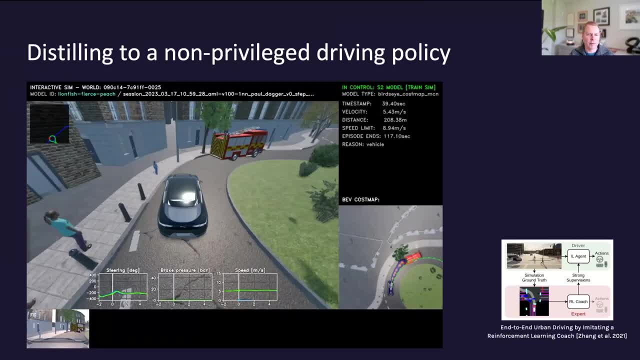 Now, it's all very well using these for evaluation and to populate our simulator for evaluation, But could we actually learn to drive from these? So far we've been talking about these, these tokenized vector representations that are privileged. They have full perceptual state about the simulation. 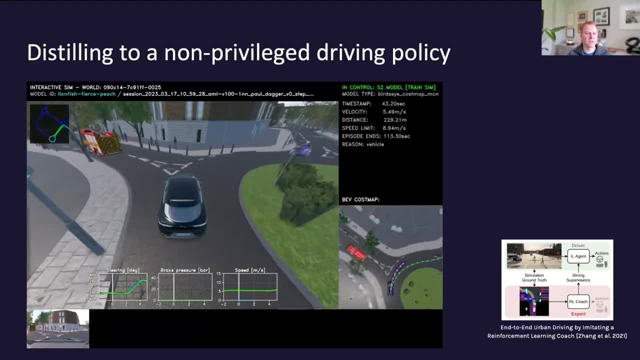 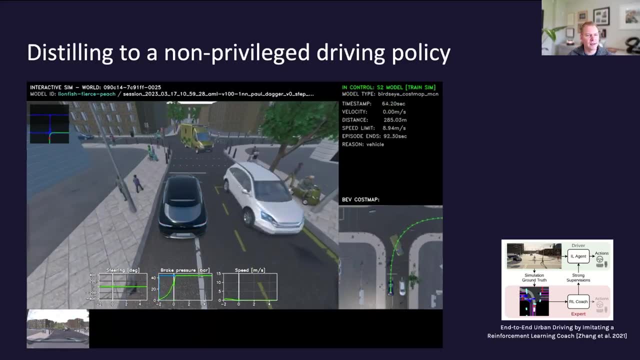 Well, can we distill that down to a non-privileged driving policy? And yes, we can, is the answer. So, using techniques similar to Zhang et al, we can take, we can learn a policy that can drive from the image that you see in the bottom left. 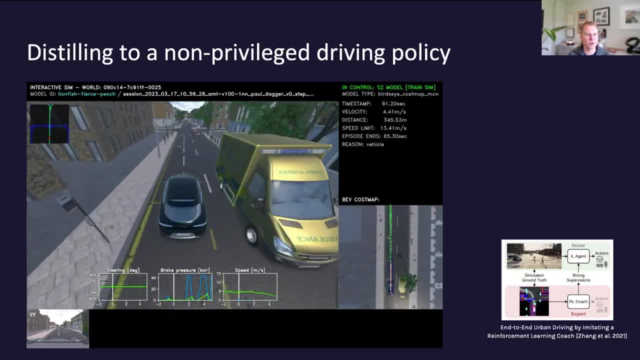 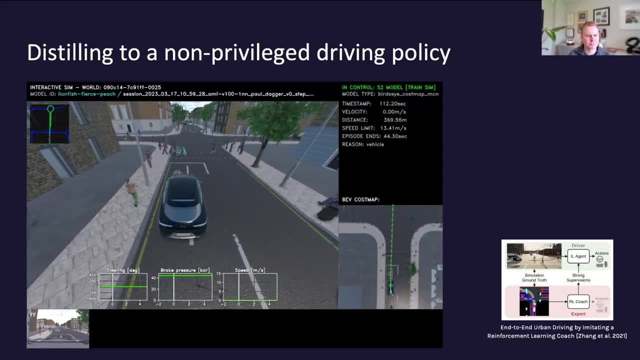 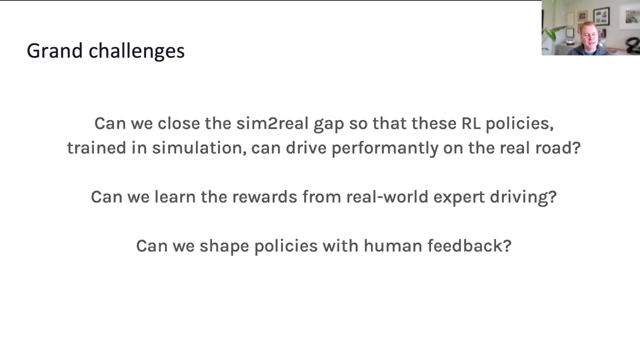 and drive pretty much as well as the as the privileged policy again in these, in these quite busy, complex urban environments. Now this has been great, but there are remain a number of grand challenges here. First of all, 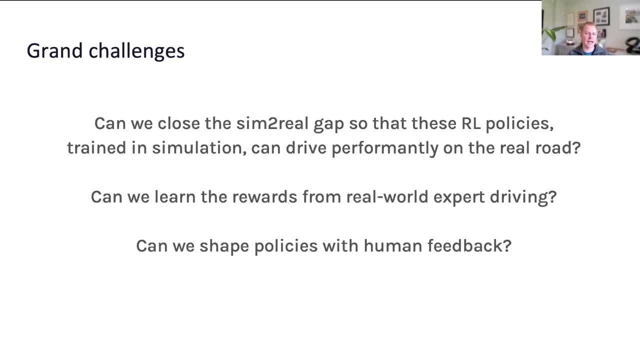 and perhaps most impactfully, can we close the sim to real gap so that these policies, these that we've learned in simulation using RL, can be taken onto the road and drive performantly? We've seen the first step of that in terms of the distillation. 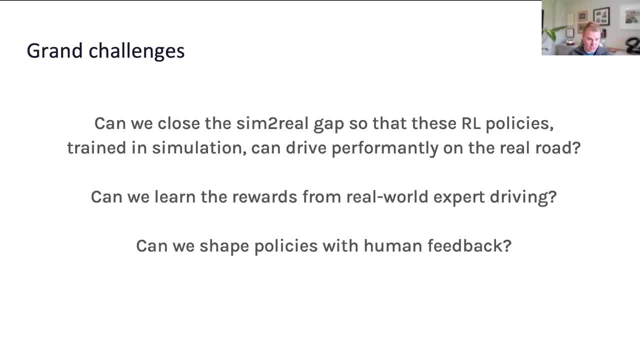 to a non-privileged policy. but can we actually take that onto the road and cross the domain gap? Can we learn the rewards from a real world expert driver? expert driving- I mean, they're pretty simple today, but is that going to be scalable? 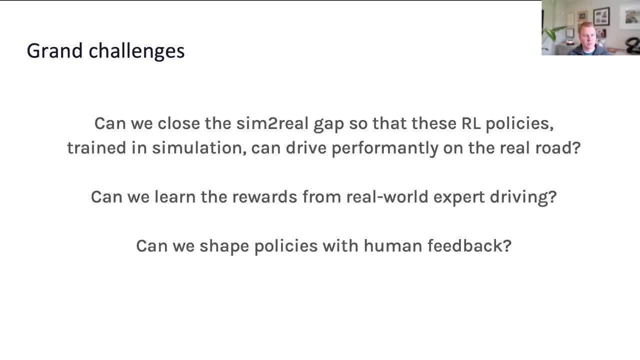 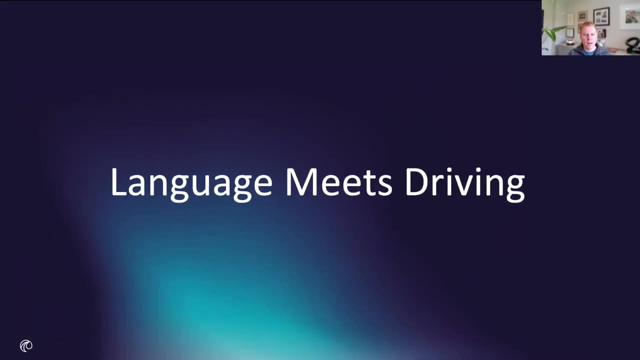 And indeed, can we shape these policies with human feedback? If we see this as learn, something that's mostly right but not quite right, can we provide human feedback to improve that? The next topic I'd like to talk about is language meets driving. 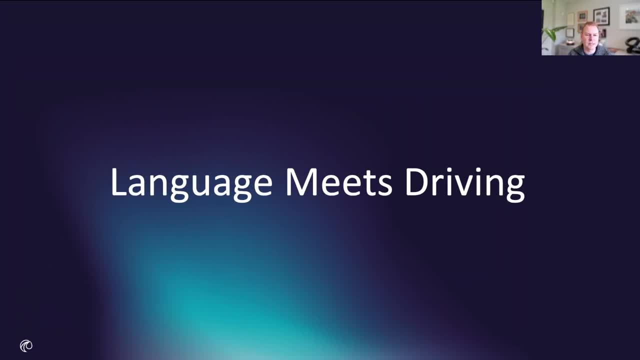 And this I'm, I'm, I'm really excited about It's- it's been amazing to see the emergence of increasingly complex understanding of language with these large language models: GPT one, two, three, four, et cetera. 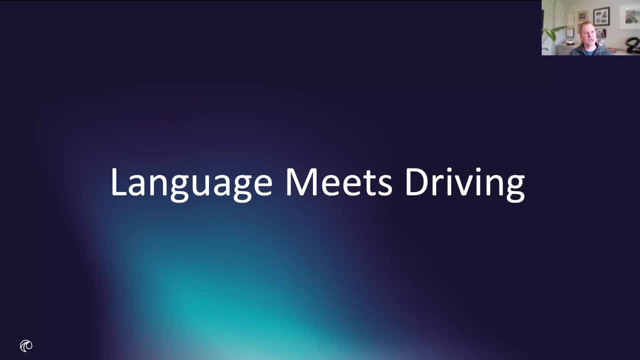 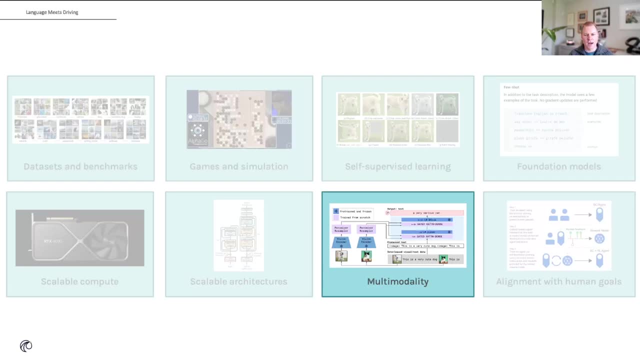 It is, but but, moreover, what's what you're starting to see now is it's not just understanding language, but it's actually understanding how to think and how to reason, And I I think the opportunity here for multimodality and bringing together 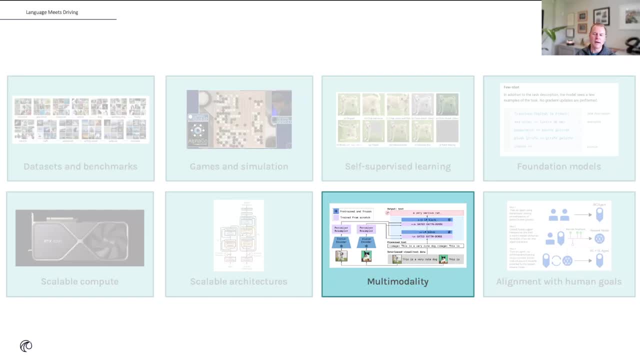 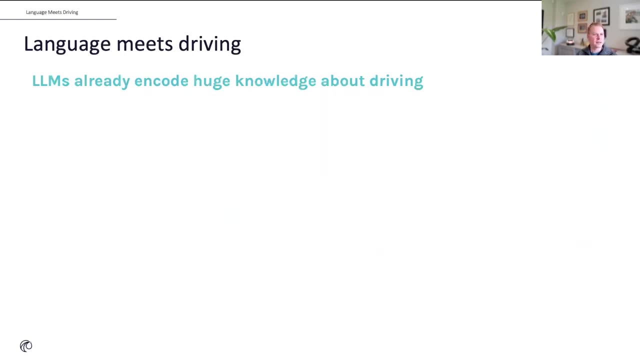 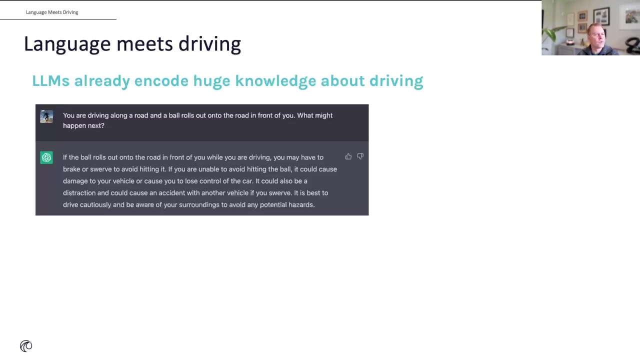 language and our, our vision. video driving and action is is potentially enormous. So let's start by looking at LLMs. out of the box, They already encode a huge knowledge about driving. So, for example, you are driving along the road and a ball rolls out in front of you. 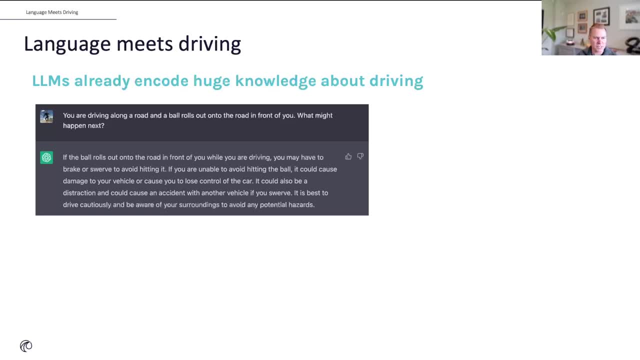 And what might happen next. Ask chat GPT and you'll get a pretty reasonable answer. If a ball rolls out into the road in front of you while you're driving, you may have to break or swerve to avoid hitting it. If you are unable to avoid hitting the ball, 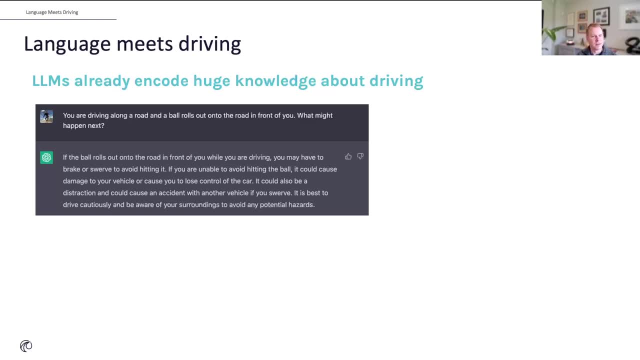 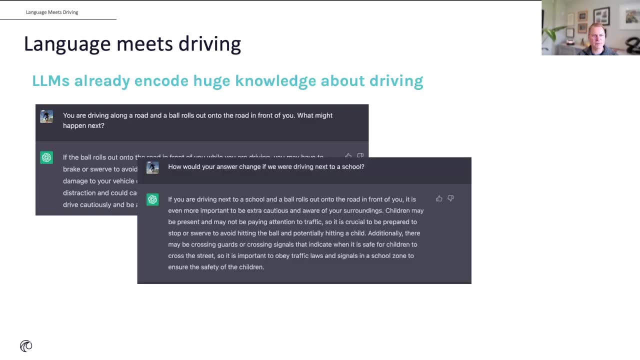 it could cause damage to your vehicle or cause you to lose control. It's best to drive cautiously and be aware of your surroundings and avoid potential hazards. So pretty reasonable answer. but you can probe it further: How would your answer change if you were driving next to a school? 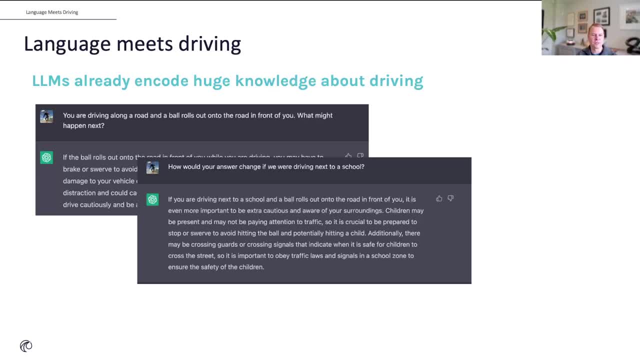 Well then, it's even more important to be extra cautious. Children may be present and may not be paying attention to to traffic. It's crucial to be prepared to stop, et cetera. Is it true Still, if the time is midnight? 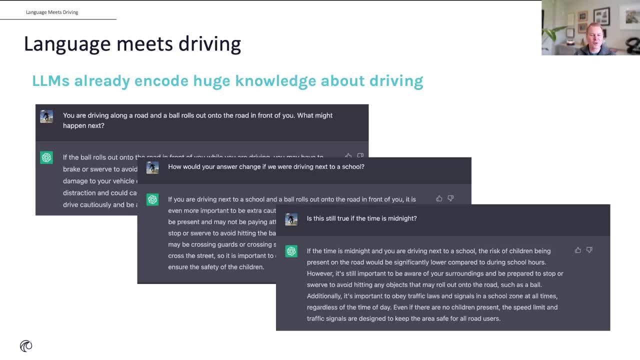 well, if it's midnight, the risk of of children being present on the road would be significantly lower, but it's still important to be aware of your surroundings and prepared to stop or swerve to avoid hitting objects. So you know. 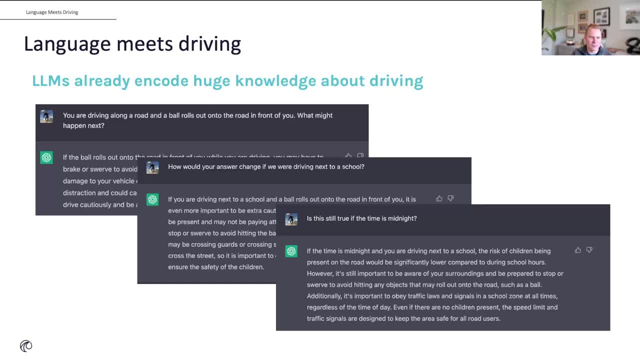 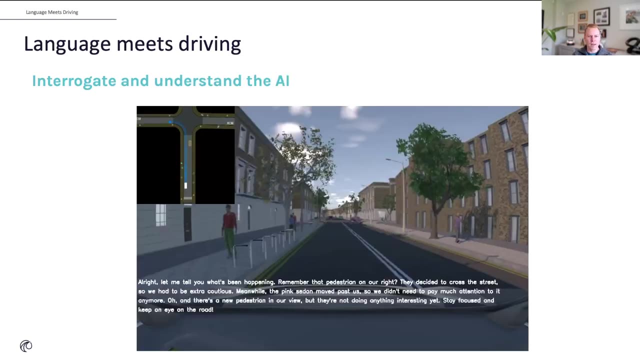 this is kind of impressive, given this is, you know, not ever seen a real road. It's. it's based purely on text, But very, very exciting that these LLMs already encode a huge amount of a huge amount of knowledge about driving. 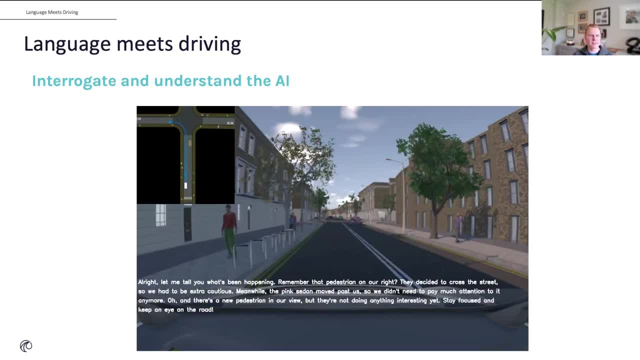 We've been starting to, to play around with this and seeing, at least as a first step, can we get, can we, can we ground language and the, the, the, the, the vision and actions that we see in the world. 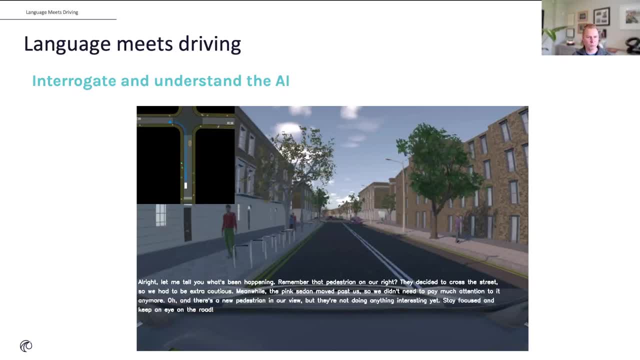 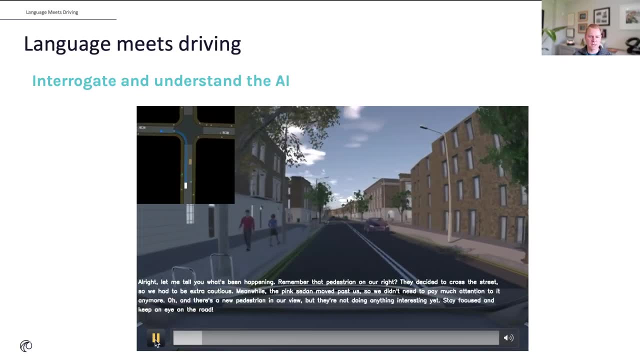 such that we can interrogate our driving models and see what it understands. And so you know, this is a little clip of driving in simulation for the moment, Where we're turning the driving into into text, And so if I pause it here, 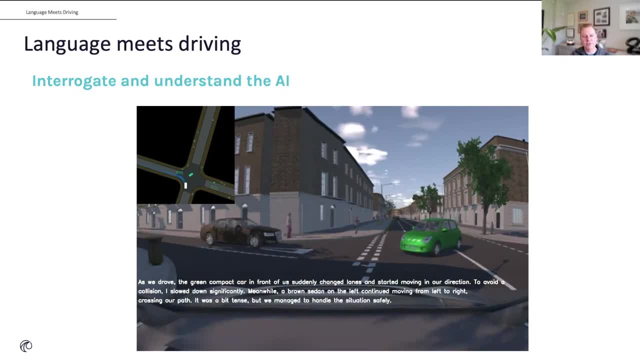 I'll read it out. As we drove, the green compact car in front of us suddenly changed lanes and started moving in our direction. To avoid a collision, I slowed down significantly. Meanwhile, the brown sedan on the left continued moving from left to right. 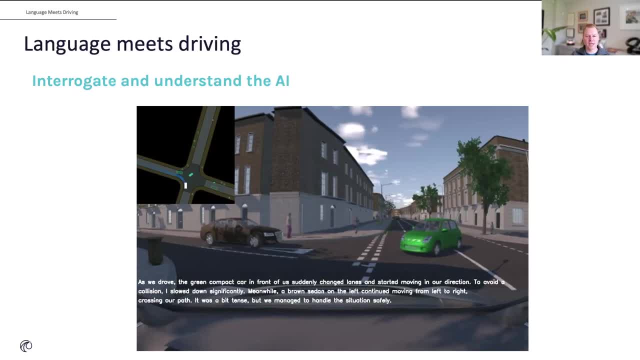 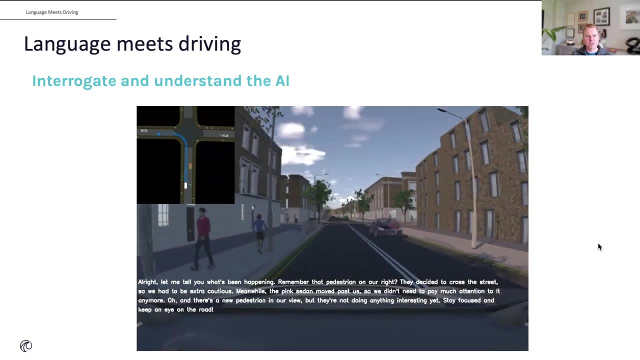 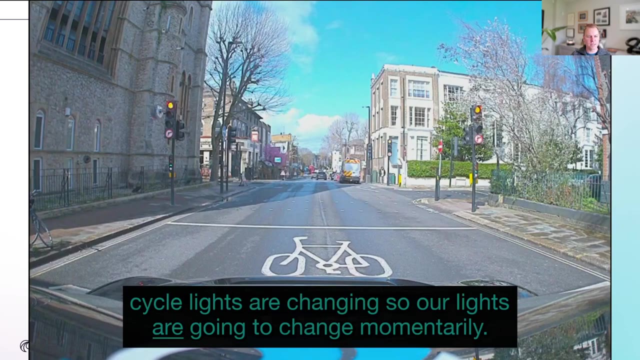 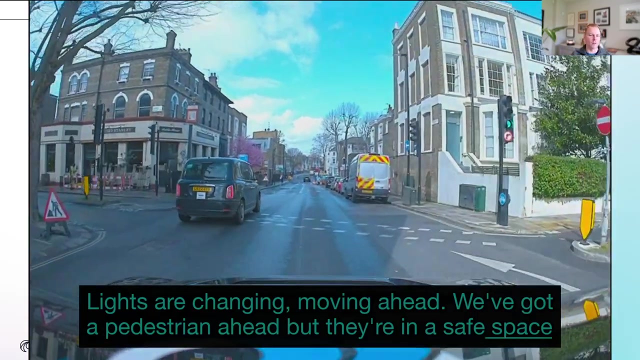 crossing our path. It was a bit tense, but we managed to handle the situation safely. Of course, we've been in simulation so far And to bridge the the the gap there, to take it to the real world, we've been starting to explore capturing a large corpus of language and driving data of the kind that you see here. 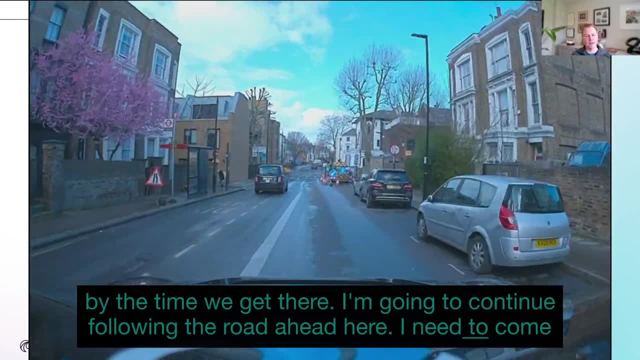 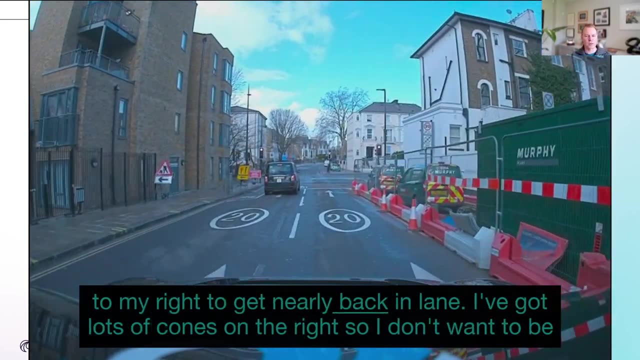 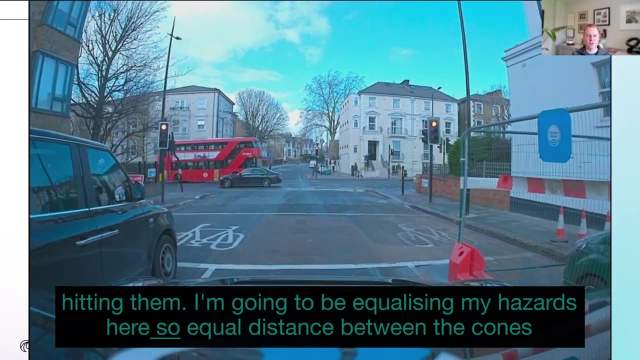 where we have our AB safety operators narrating as they as they drive and describing the scene in quite a lot of detail about what's going on, What are the important things to pay attention to, What are the causal factors of decision making, et cetera. 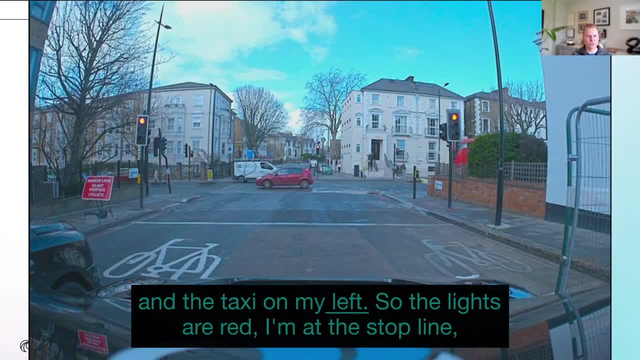 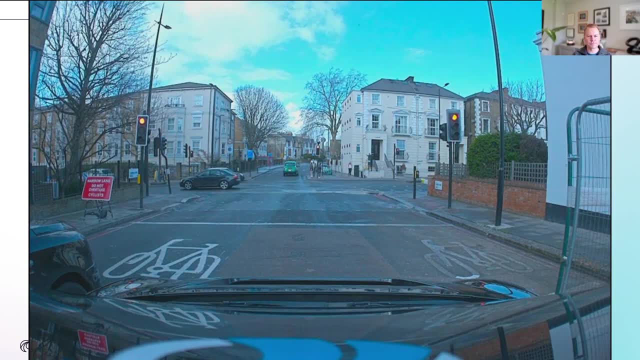 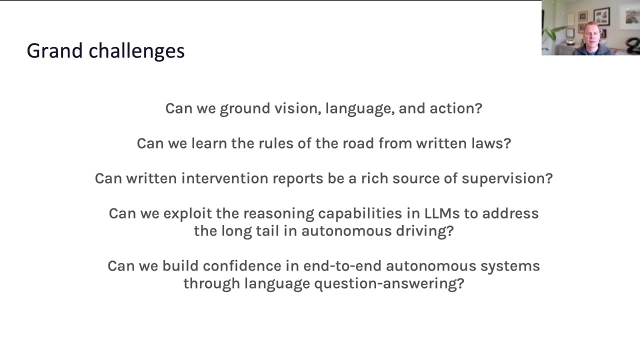 We believe that this, this dataset, is going to be a phenomenal resource to enable us to explore vision and language grounding. So the grand challenge is here: Can we actually do this? Can we ground vision, language and action? Can we learn the rules of the road from written laws? 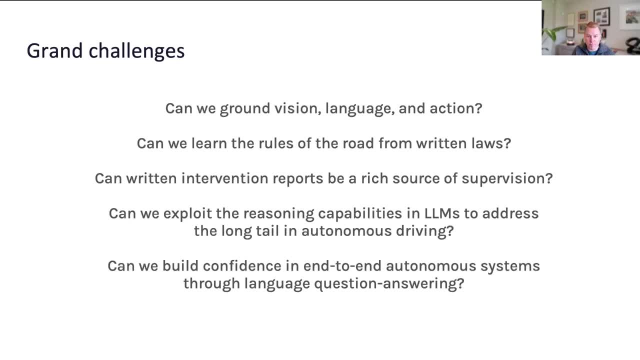 right. In the UK at least, there's a, a book that literally writes down the rules of the road. If you could do that, that gives you enormous. you know rapid means to learn from those written laws. Could you use intervention reports written in natural language to be a source? 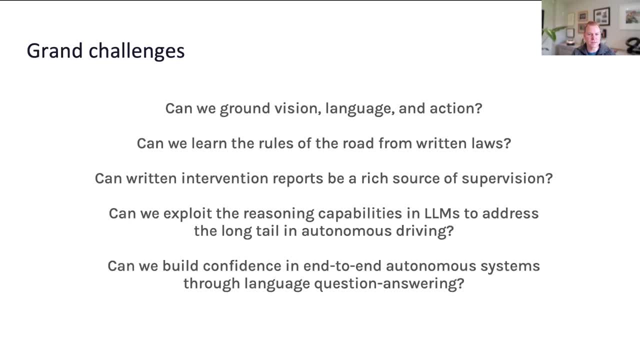 a rich source of supervision which again perhaps tease out the causal factors of what went wrong and why it should have done something differently. Can we exploit the reasoning capabilities that these LLMs seem to have to address the long tail, And can we build confidence? 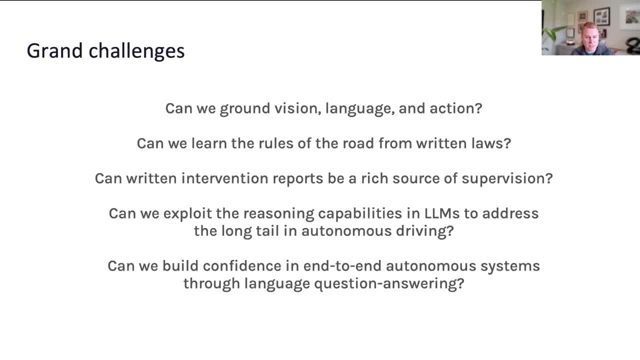 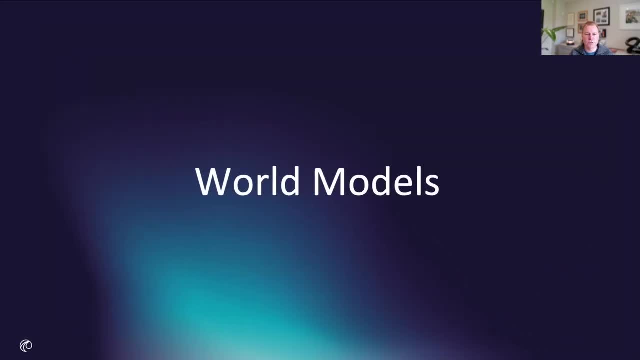 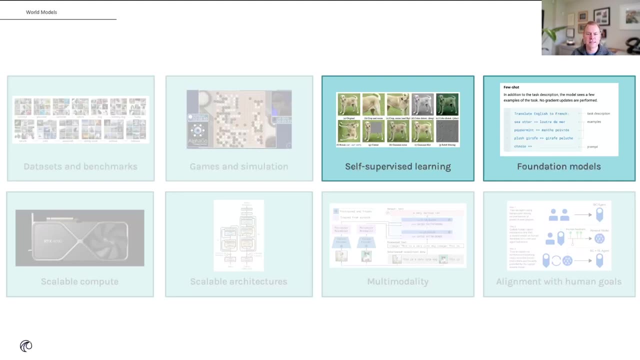 increasing confidence with end-to-end autonomous systems through language Q and A. The final section I want to talk about is world models, And this very much aligns with the themes of self-supervised learning and towards foundation models. So it's pretty clear to drive well. 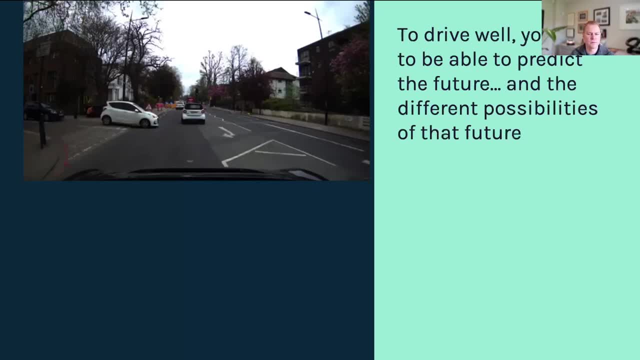 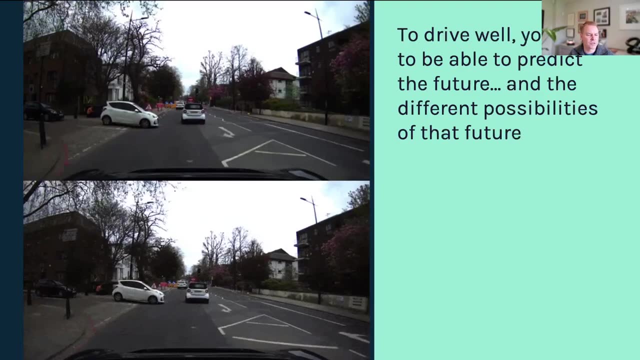 you need to be able to predict the future and the different possibilities of this, of that future. So this white car, is it stationary? Is it in the middle of a turn? What's it going to do Now, if I show you a video? 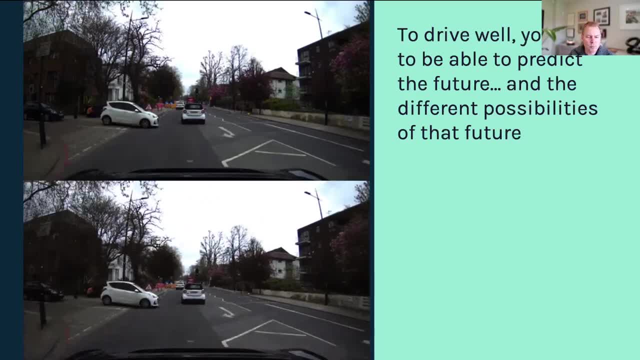 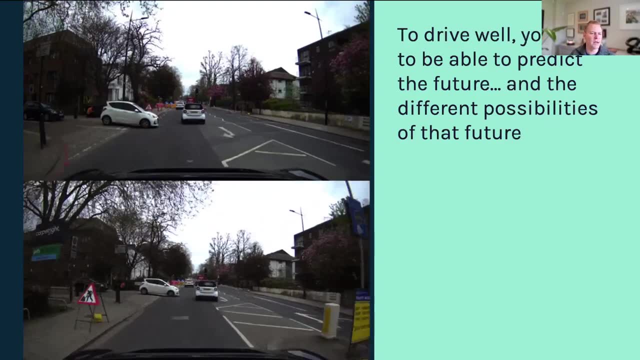 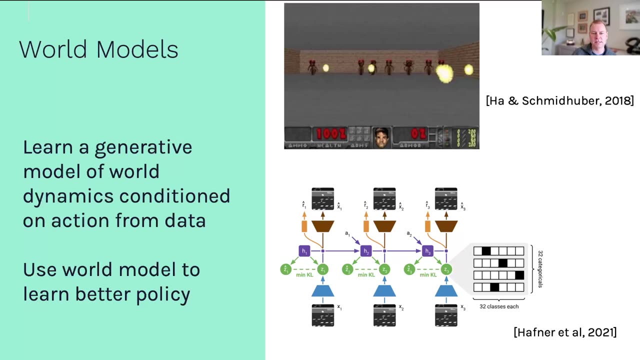 it's a lot clearer that it's actually pretty stationary here, but it still could. There is a possible future where it pulls out suddenly unexpectedly, And it is important to be aware that that is a possibility. World models have been an exciting topic of late. 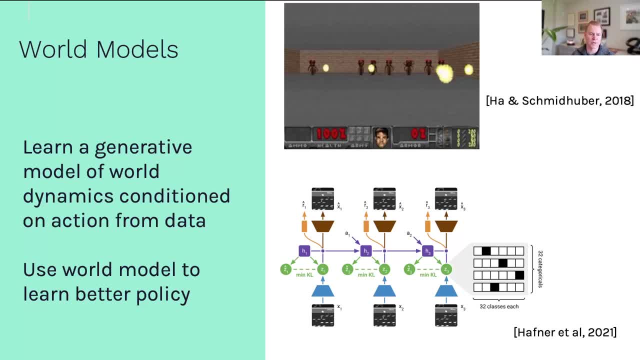 Basically, you know, a lot of work has focused on games and learning a generative model of the world dynamics conditional action from data within these games And then using that world model, that world dynamics model, to learn a better policy through. 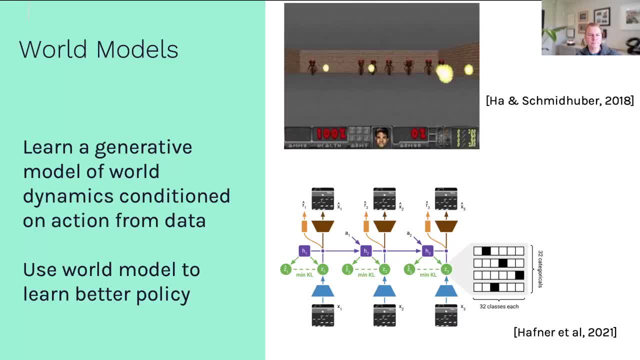 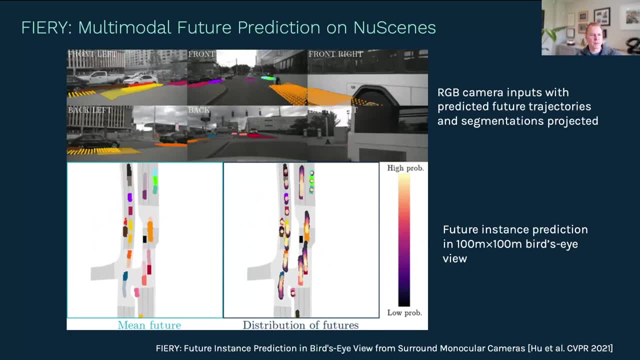 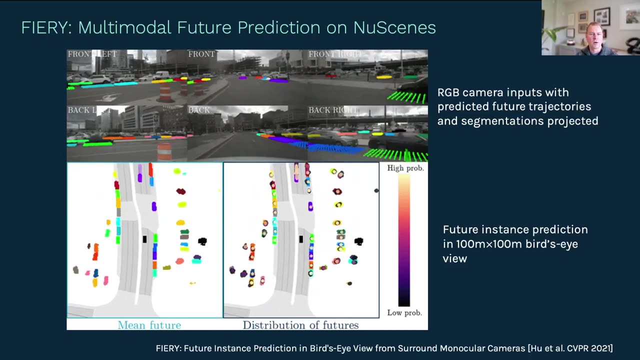 for example, model-based reinforcement learning. We've been excited about this topic for a little while now. The last couple of years we've been working on various aspects of world models, So our CVPR 21 paper called Fiery worked on the new scenes dataset. 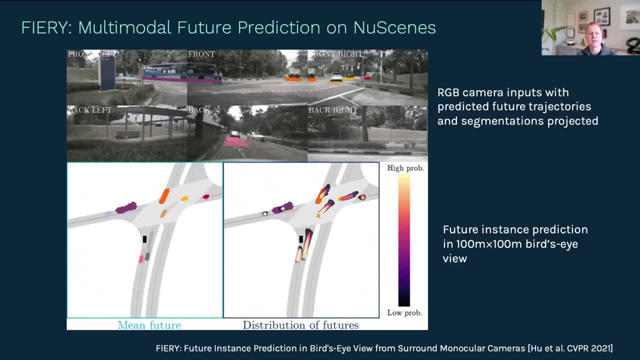 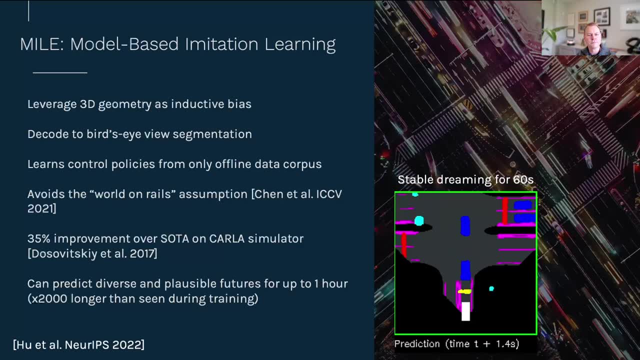 and aimed to predict the future evolution, the multimodal future evolution, of driving in the scene. More recently, our work MILE at NeurIPS last year. model-based imitation learning used 3D geometry as an inductive bias and allowed us to build control policies from offline data corpora. 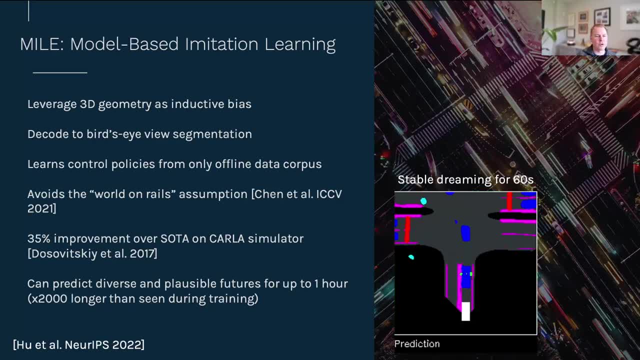 that avoided the world on Rails assumption. So the world on Rails assumption improved the state of the art on the color simulator and was able to predict diverse and plausible futures for up to an hour in the future And you can see a bit of an example of stable dreaming. 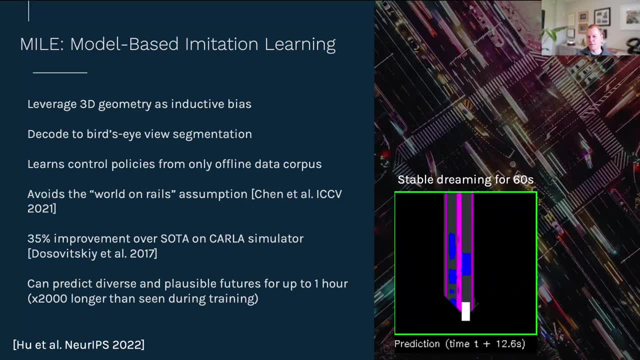 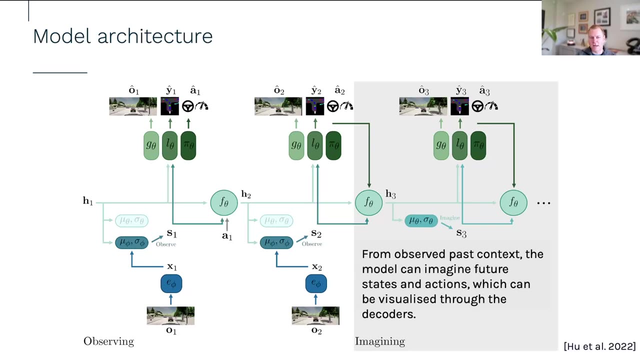 from this model. on the right there, That's a top-down view, where the white is the ego vehicle, the blue are the imagined vehicles ahead the red there is a traffic light that then turns green, et cetera. This was a fairly interesting autoregressive architecture. 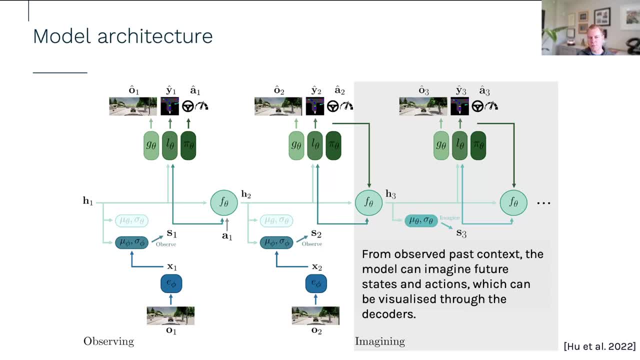 where you could essentially unroll, encode from observation, decode back to another observation or to the bird's eye view representation and unroll, if you want to, to dream into the future, And so again we could see multimodal predictions. 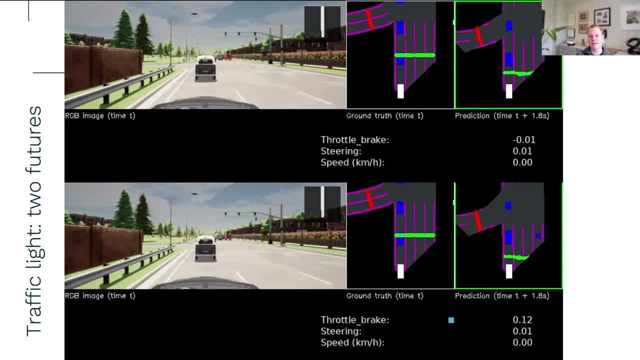 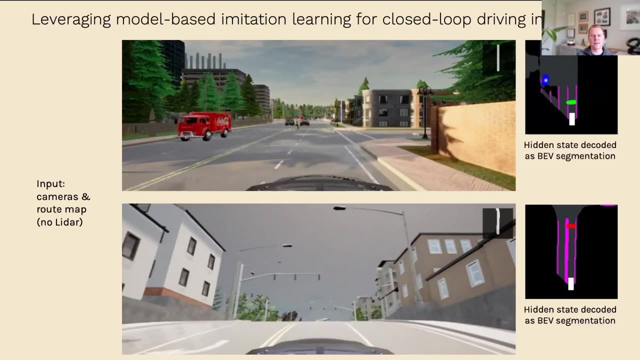 And here the top row shows an example where the traffic light turns red in its imagination and the ego vehicle stops. The bottom row shows the vehicle continuing through the light And of course, we can then drive around in the simulator using this. 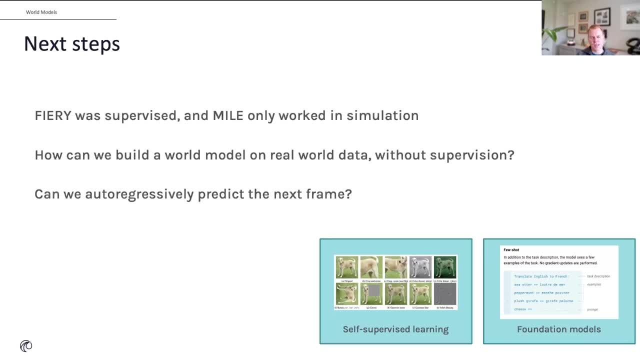 and this improved our driving performance. But Fiery was a supervised approach and Mile only required our simulator required to work in simulation. How can we build a world model that works on real data without supervision? And you know, taking a leaf out of the large language models book, 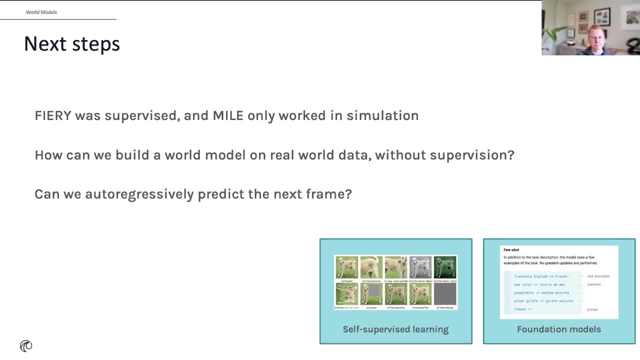 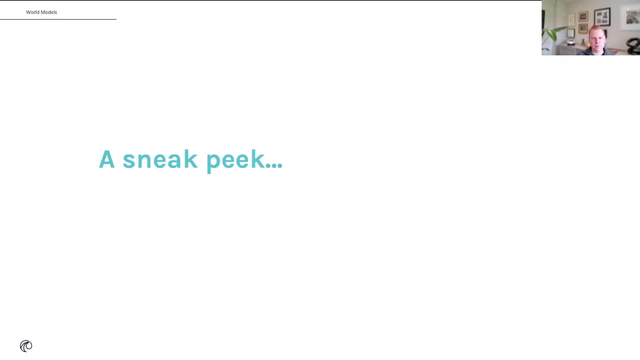 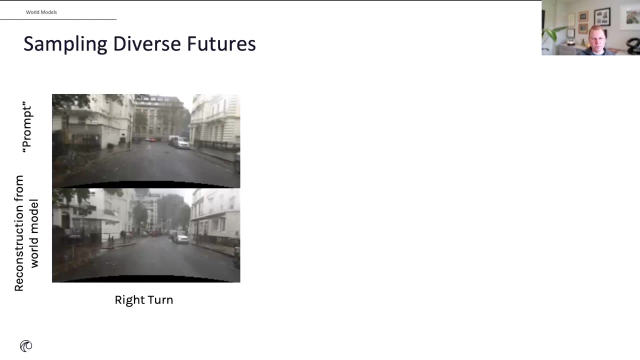 can we autoregressively predict the next frame? And well, the answer is yes, And I'm going to give you a very quick sneak peek of something that we are incredibly excited on and iterating rapidly. This is a unsupervised, a self-supervised world model that we've 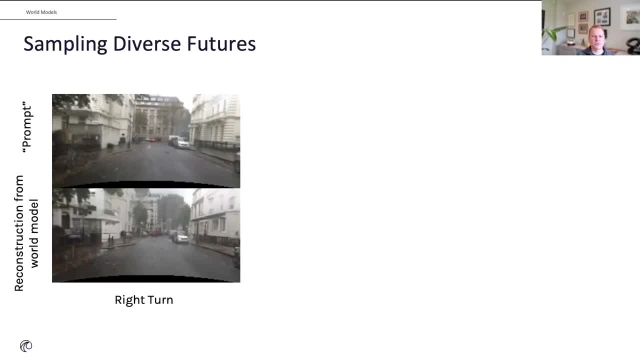 we've generated and it's going to imagine a driving situation. So the, the top, you see the, the prompt for sort of two seconds, the conditioning, and then the bottom. it's going to imagine what's going to continue in the scene as a full. 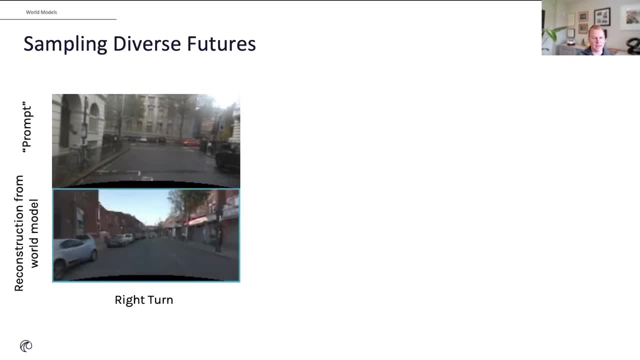 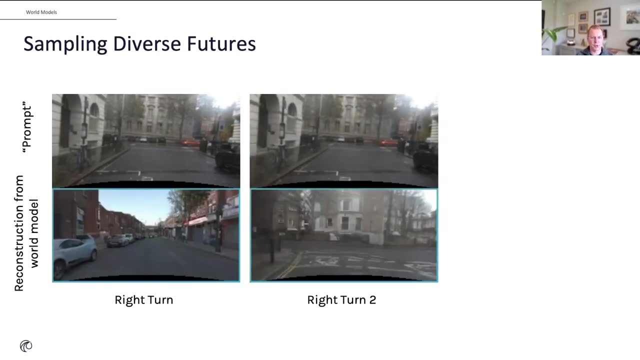 a full video And it's imagined, a right turn. Well, we can move on and do the same again, do another sample from this generative model And this time again we do a right turn. but you'll notice that the 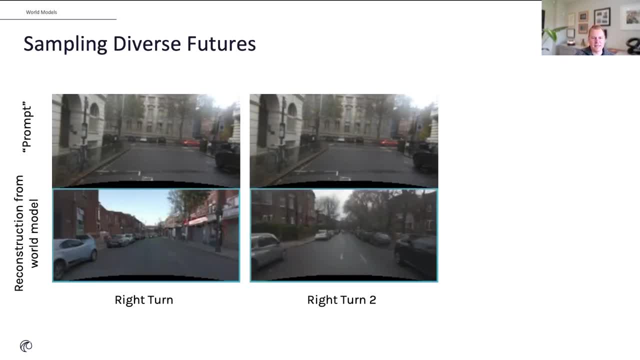 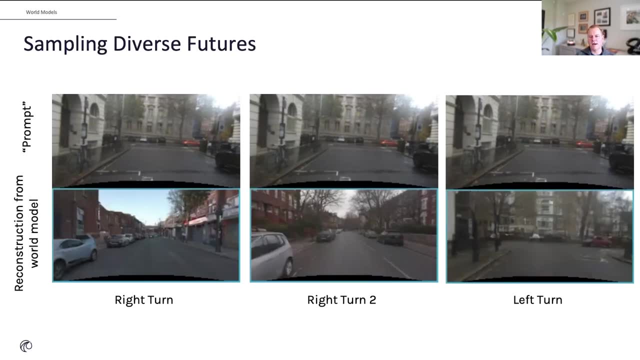 it imagines something completely different, a completely different street scene. So you know, yet again let's do another sample, And here it's going to imagine a left turn. We're not conditioning it, It's just deciding to do a left turn when it gets to the end of the road.